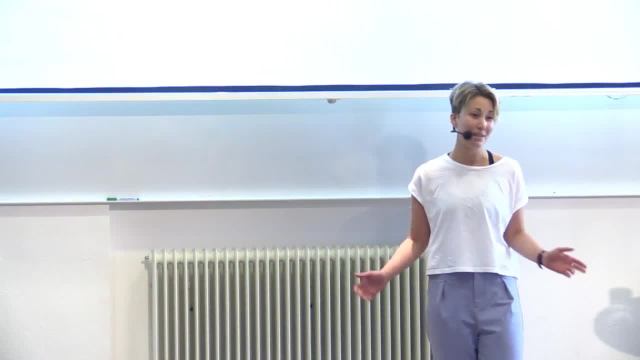 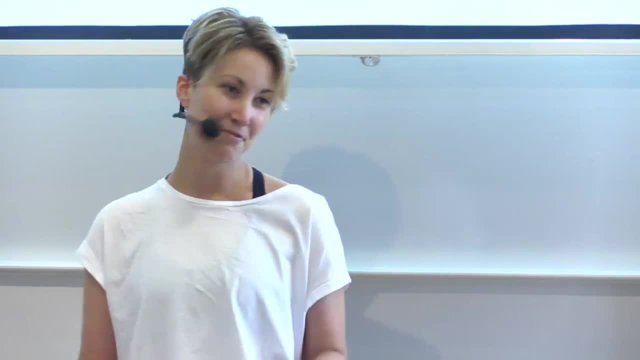 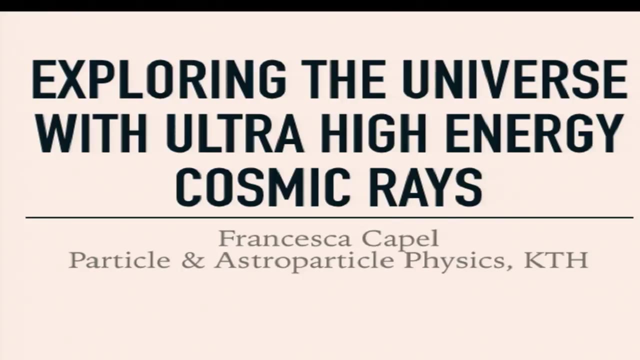 I'm not an expert- that's been in the field for some 20 plus years. With that in mind, what I want to do today is give a fun and informal introduction to my perhaps unusual area of research that I found to be a very rich and fascinating corner of physics to work in for the past three years now. 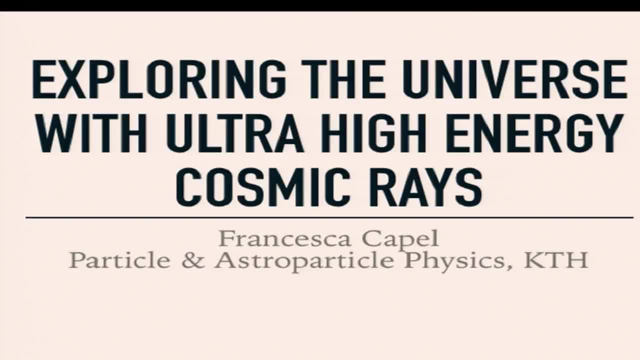 The title of my talk is Exploring the Universe with Ultra-High-Energy Cosmic Rays. I think the first part of the talk is going to be a little bit about the universe itself. The title is kind of self-explanatory. Physicists are often exploring the universe. That's kind of their job. 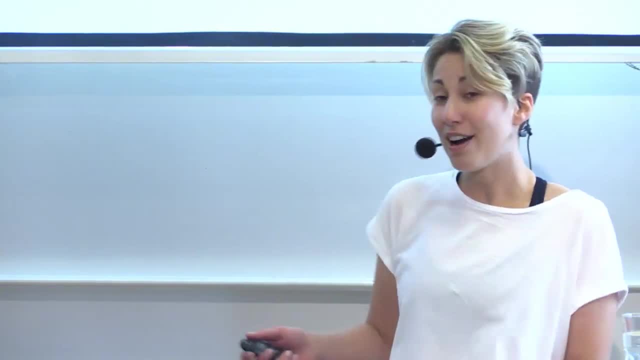 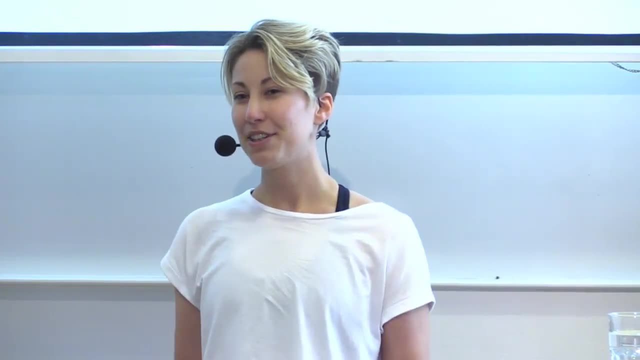 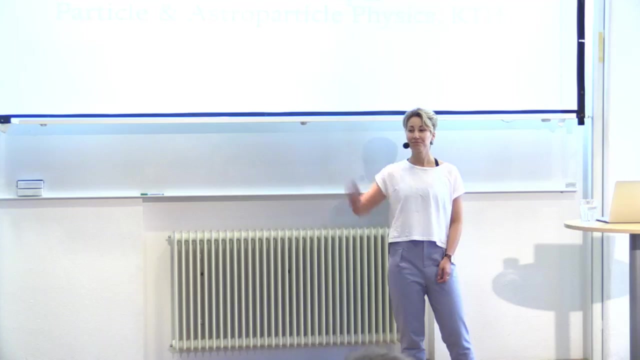 And I think, following on with Ultra-High-Energy, you can kind of understand what I'm getting at here, But I don't really know the kind of level of the audience, And so I wanted to ask who here knows, or thinks they know, what cosmic rays are. 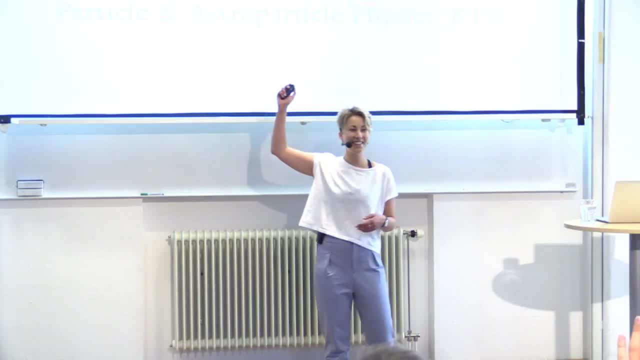 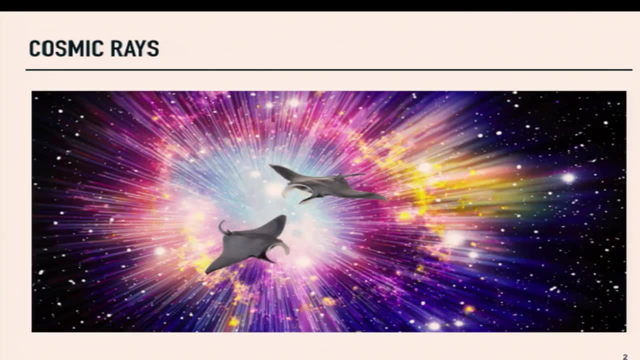 Just raise your hand. I know what they are, so we're going to be okay, All right, All right. So this is a few, So I'm going to start with cosmic rays, right? So whilst I think that some kind of space-traveling manta rays would be a great basis for a talk, 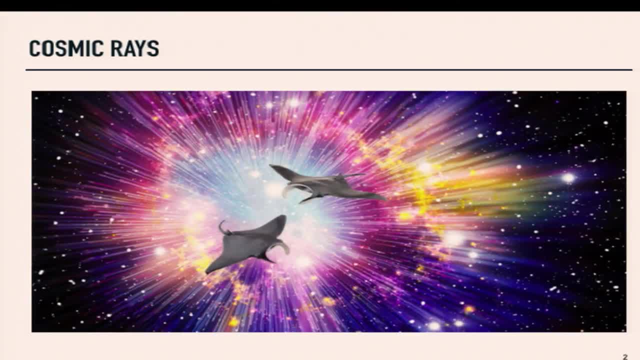 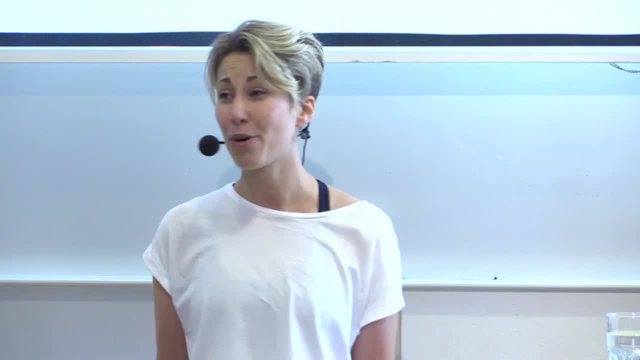 and perhaps an even better movie idea. this is not what cosmic rays are, And kind of on a more serious note, what I really wanted to say here is that the term cosmic rays is somewhat ambiguous, And this is because, when they were discovered, people didn't actually know what they were. 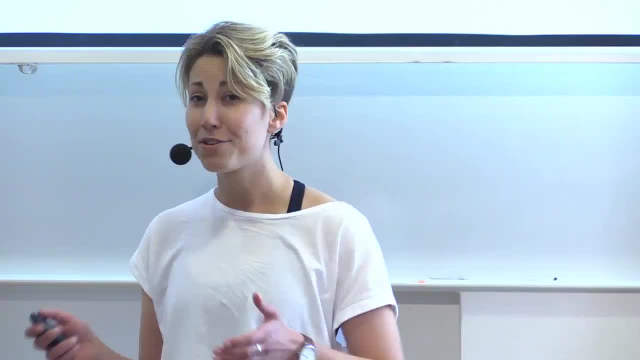 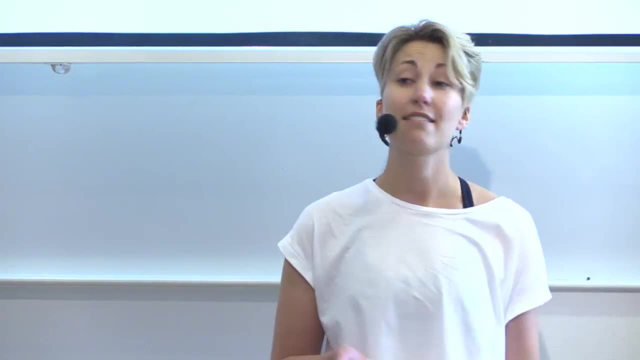 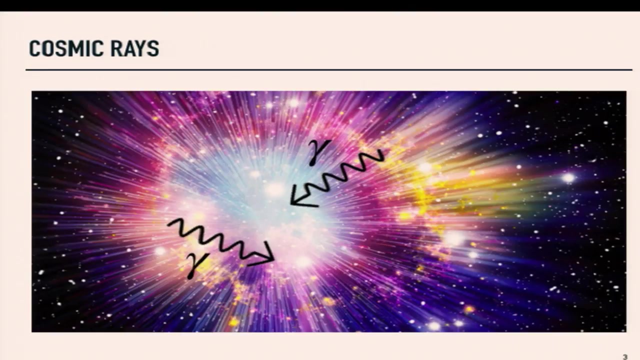 just that. it was some kind of radiation of unknown non-terrestrial origin. So rays are typically associated with electromagnetic radiation. so photons- We have words like gamma rays, X-rays, that physicists are quite familiar with. But what I'm going to be talking about today, and what the word cosmic ray means in kind of the modern research area, 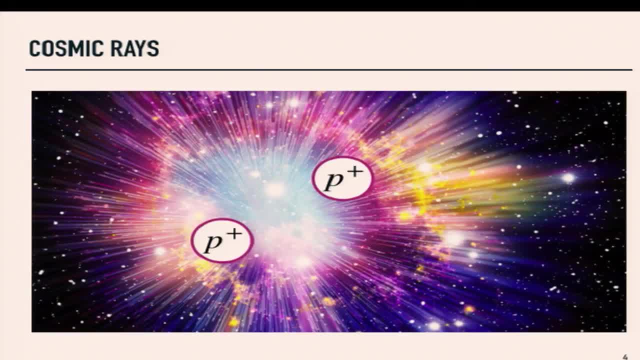 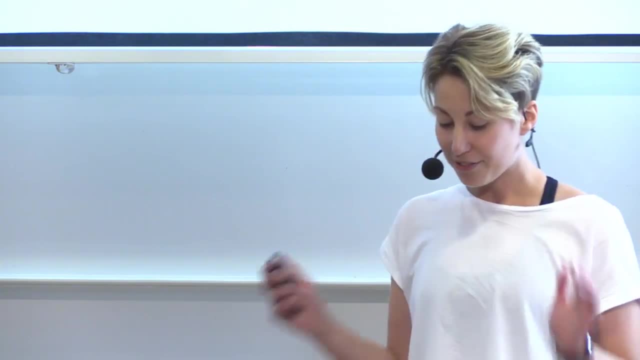 it's actually very energetic, massive charged particles, For example positively charged protons, or indeed even heavier nuclei that have been ionized, like helium, oxygen, silicon, iron and so on. So these are quite different things and I just wanted to get that straight kind of before I continue in the talk. So I'm going to start with some history. Cosmic rays were discovered by Victor Hess over 100 years ago now, in 1912.. And I've said discovered here because, like kind of any science, scientific discovery, it's hard to really attribute that to one person. 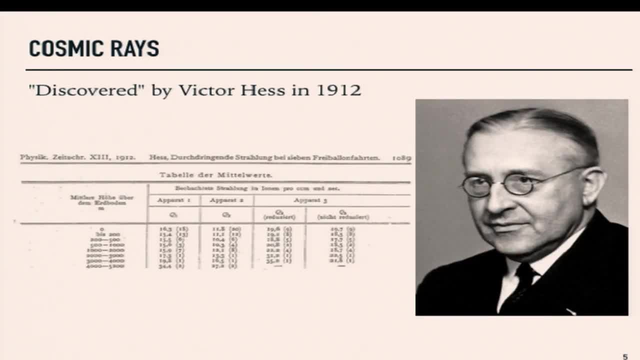 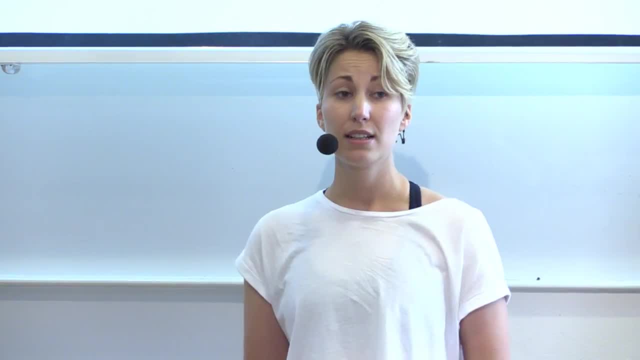 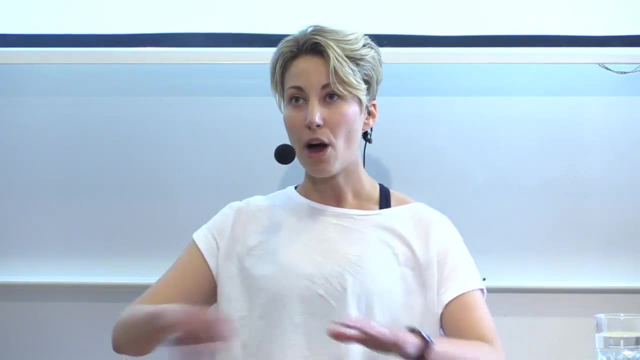 But that's kind of what happens. But what was really going on at the kind of time that Hess was doing research was that scientists were doing experiments with electroscopes- So these were kind of old school radiation detectors basically- And what they saw was that there was kind of this ambient radiation they could detect. 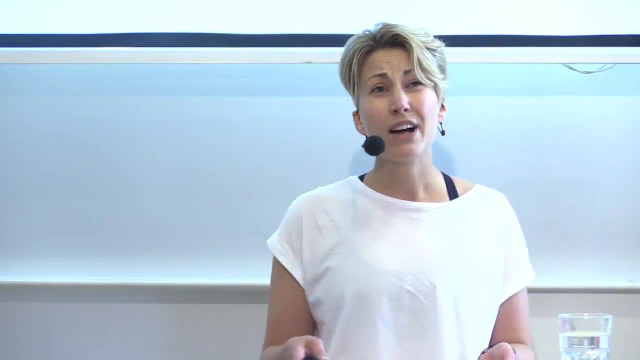 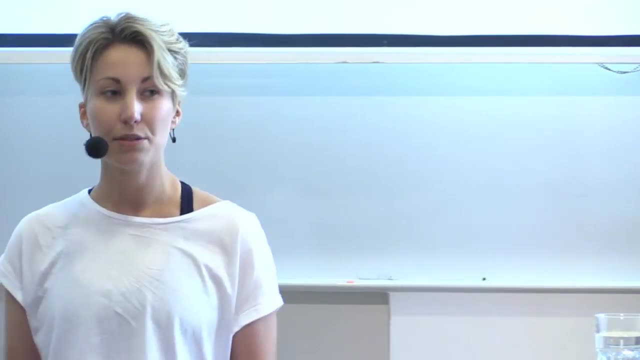 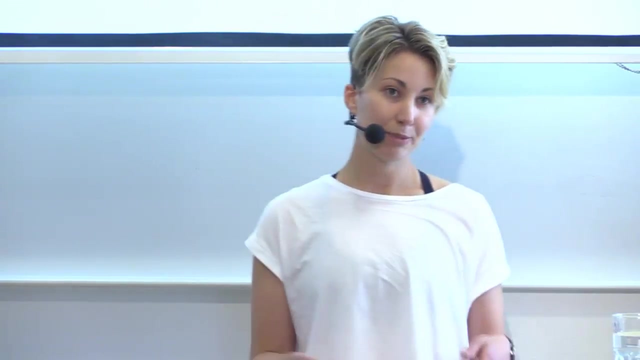 that didn't really seem to be coming from anywhere And the working hypothesis was that this radiation came from the Earth And people kind of backed this up by going underground and they could still see reasonable signals in their radiation detectors. So what people wanted to do to test this hypothesis? was to actually move away from the Earth, so go up, And the idea was that if you did that, then the amount of radiation that you see is going to decrease, And so I think one of the first people who really tested this was actually called Theodore Wolff. 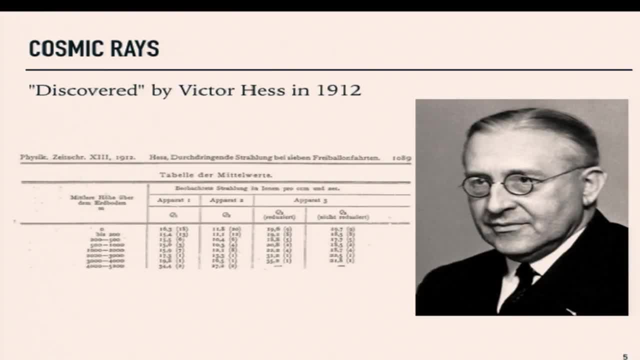 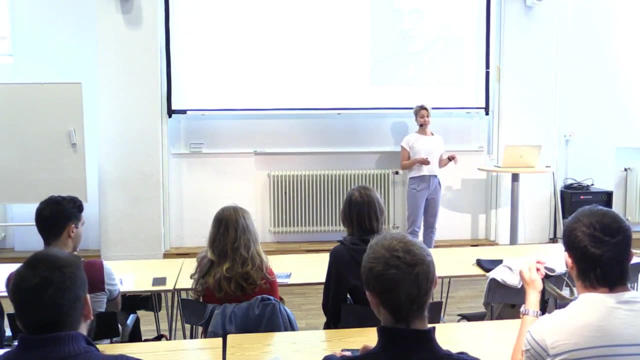 Slightly before Hess. in 1910, he took an electroscope to the Eiffel Tower in Paris and measured the radiation level at the bottom and the top of the towers. That's about 300 meters height difference, And what he saw is that the radiation level did decrease. 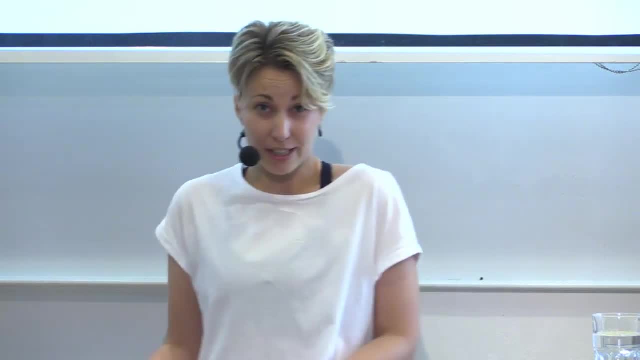 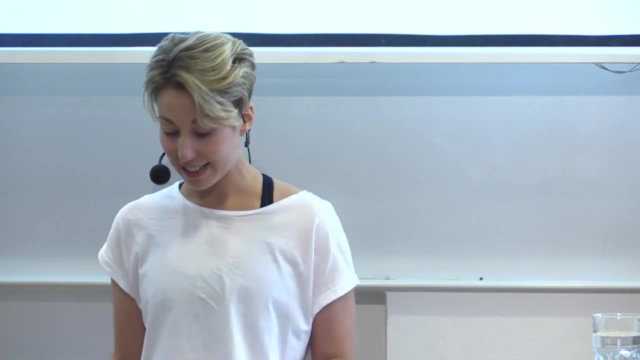 but not even slightly as much as people thought that it should. in current theories, This was kind of still an interesting and inconclusive result. So then, what Hess did was kind of go one up and he took three different electroscopes on a series of hot air balloon flights. So he managed to go much higher, up to several kilometers in the atmosphere, and measured the radiation level And his findings were published in 1912.. This is the table And you can see that there's kind of height here in one column. 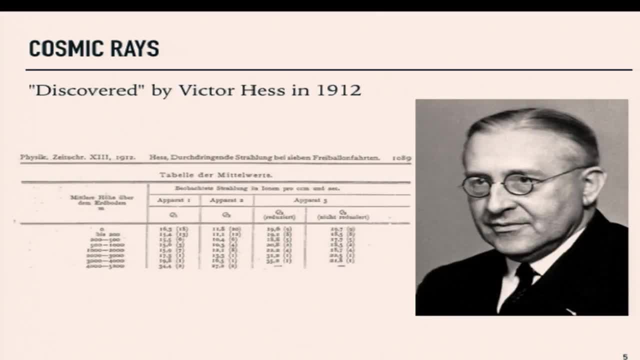 and then radiation level in three different detectors. But I think if Hess had had access to kind of modern technology and a love of data visualization like I do, his results might have looked something more like this. So what I'm showing is the same table, basically. 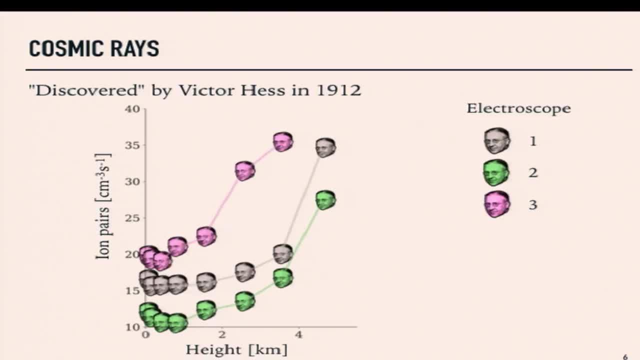 with radiation level on the y-axis and height on the x-axis, And the little different colored Hess faces correspond to the different electroscopes that he used. And what he saw in all three detectors was that as you ascend there is indeed a kind of dip in the radiation level. 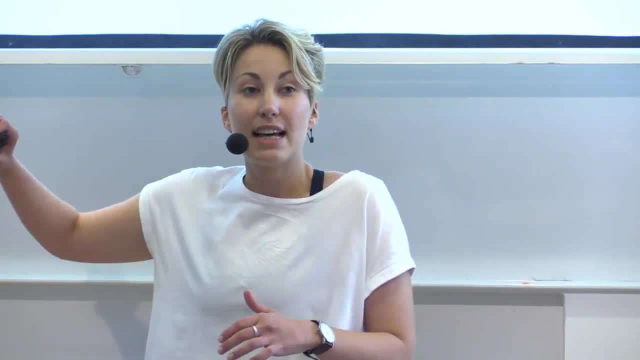 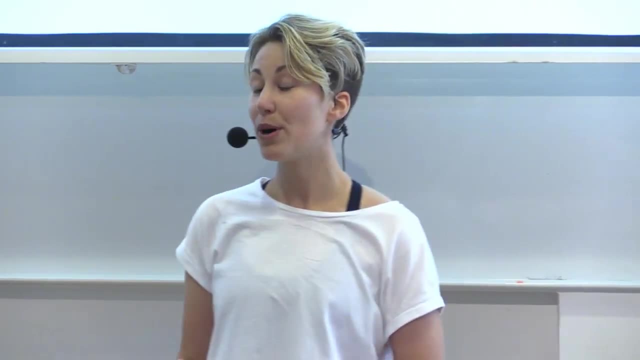 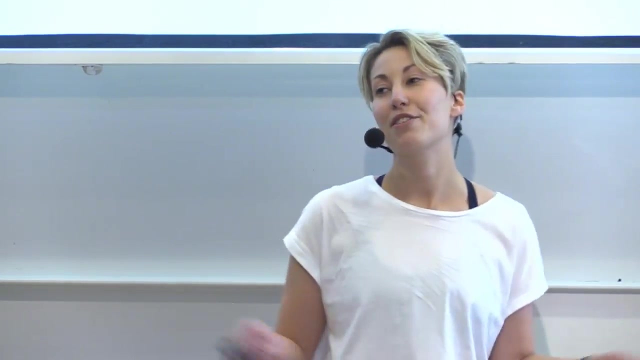 like right at the start here, But then as you continue to ascend, the amount of radiation he detected dramatically increased And kind of the obvious conclusion of this work was that the radiation can't be of terrestrial origin and it must be coming from some unknown cosmic origin. 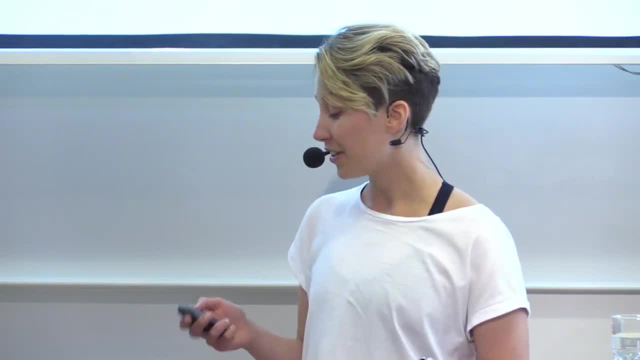 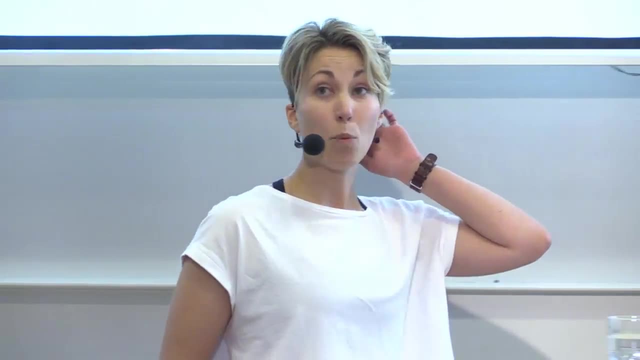 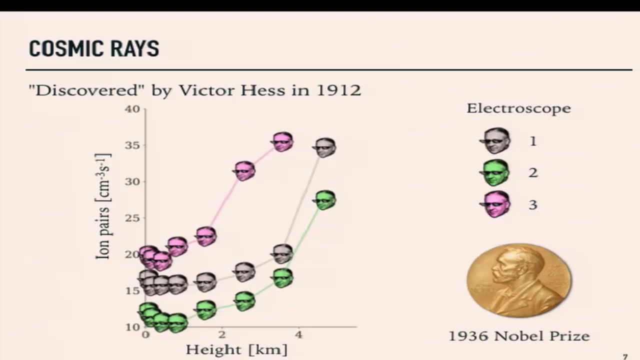 and hence the term cosmic rays. So after this discovery several scientists then followed up on this work and repeated the results and it eventually became widely accepted in the field And Hess actually got the Nobel Prize for this discovery in 1936.. So I really like this story because it's still 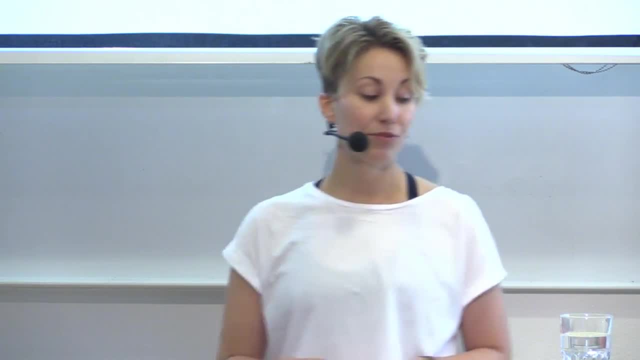 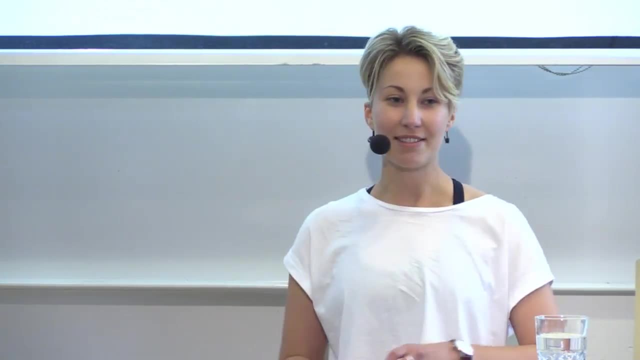 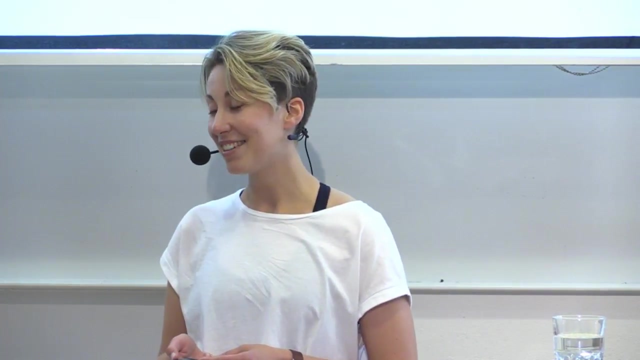 and kind of throughout the history of cosmic ray physics and still very much today. it's really common that we see unexpected results and that we change our thinking quite dramatically, But we still don't know where they come from, especially at the ultra-high energies. 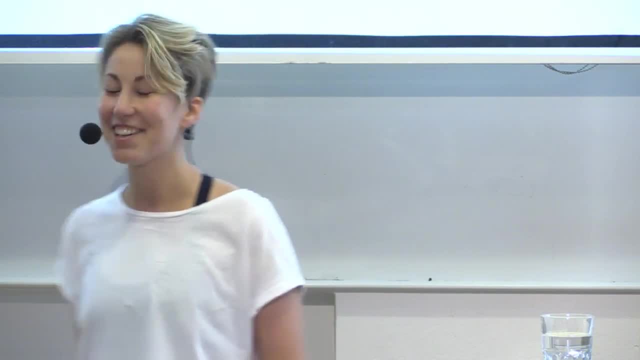 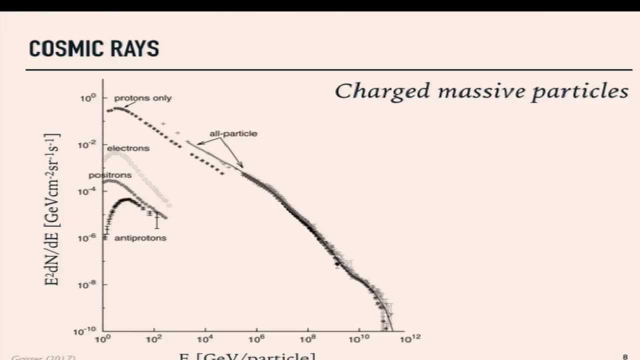 So in some senses it feels like not much has changed in the last few years, But some things have changed. Today we have a lot more data. I'm going to try and summarize all cosmic ray data in one plot, And this is what we call. 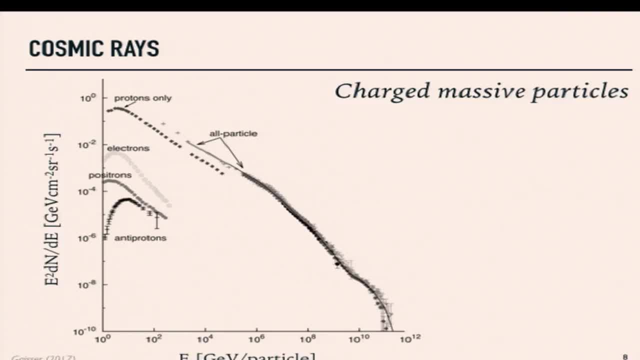 the energy spectrum of cosmic rays. So it's really just flux on the y-axis. So this is the number of particles, or kind of how common they are, And then on the x-axis is energy. So what we see immediately is that first, 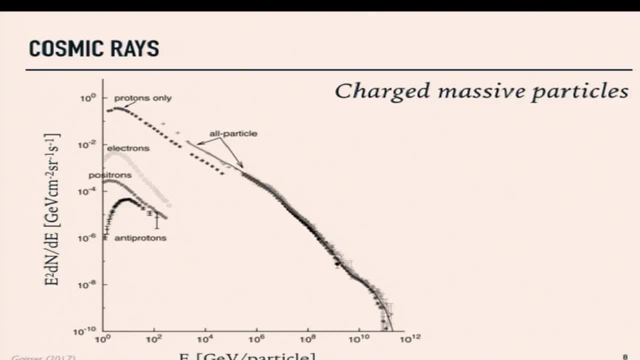 the number. I've realized my slide is coming off a bit, but this is energy. What we see is that the cosmic ray kind of physics, its spectrum extends over many orders of magnitude in both flux and energy And the kind of second thing you notice. 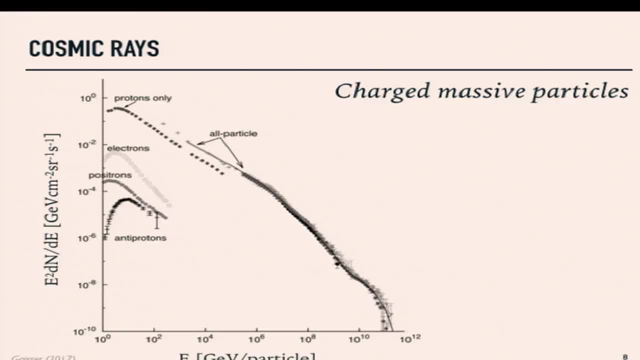 is that it's kind of doing roughly the same thing along the whole spectrum. So this is a logarithmic plot And so this line in logarithmic space is kind of mathematically described as a power law And the little bumps and features and shapes. 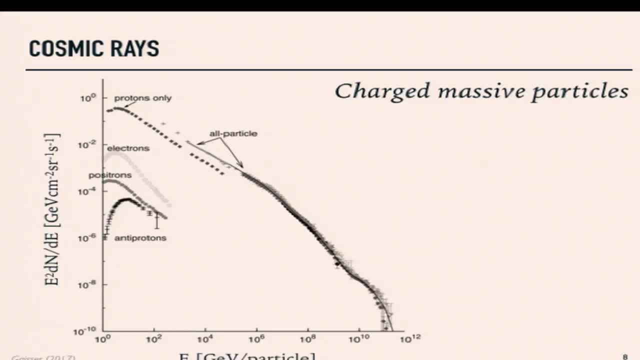 that we see in this power law allow us to kind of connect to and interpret the underlying physics of these particles. So the energy spectrum is kind of core to the study of cosmic ray physics And it's commonly referred to in the literature and in the field. 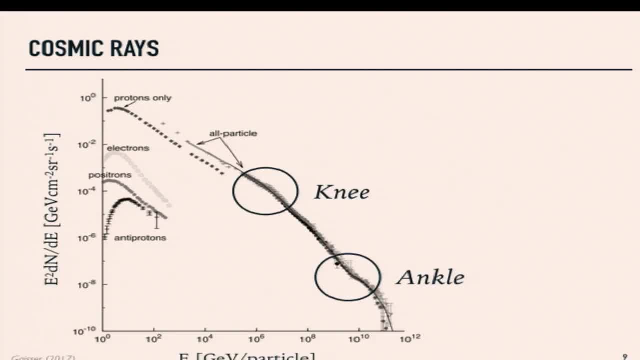 as a leg. So these two big features that you see here are called the knee and the ankle. I think that's going to be really confusing for people that are not familiar with the field when they pick up a paper and see these words, And even more confusingly. 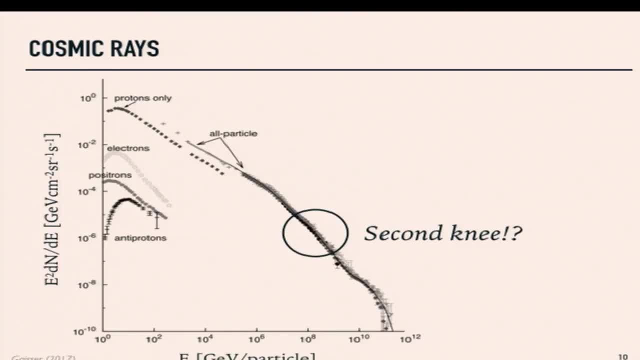 there's now a proposition of a second knee, So the analogy is kind of breaking down there. So because of the shape of this spectrum, the vast majority of cosmic rays are at the lowest energies, And the lowest energy cosmic rays we believe to come from energetic processes in the sun. 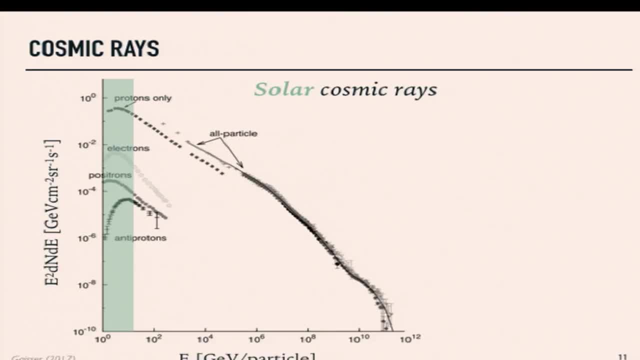 So they get accelerated to these somewhat energetic states And then, moving up in the spectrum, we have the imaginatively named high energy and very high energy cosmic rays, And these are believed to come from kind of energetic events in our galaxy And at some point in between high and very high energy. 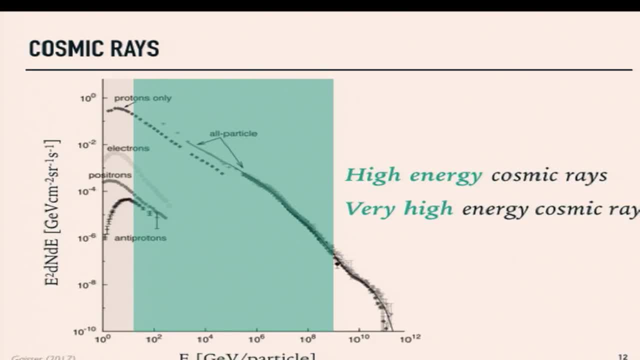 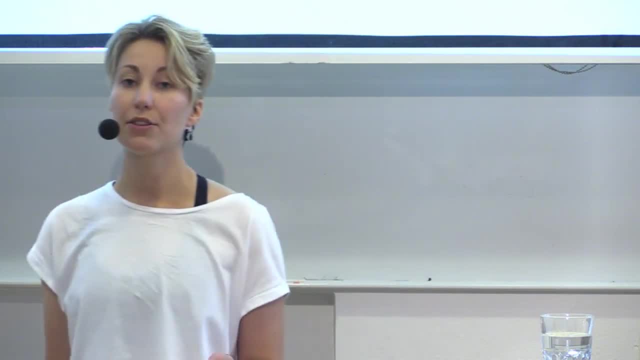 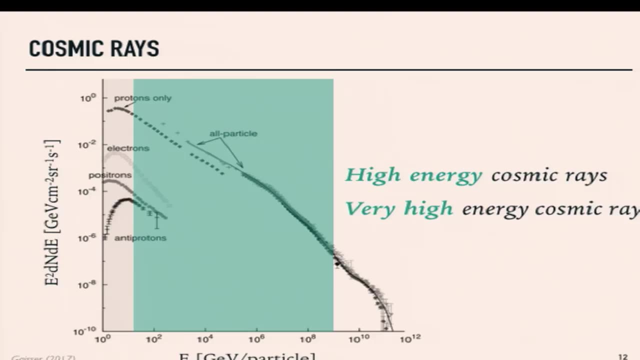 maybe at the knee, maybe at the second knee, maybe at the ankle. it's hypothesized that we should have a transition from galactic to extragalactic cosmic rays, Simply because as you increase the energy of these particles, it just gets harder to confine them in small spaces. 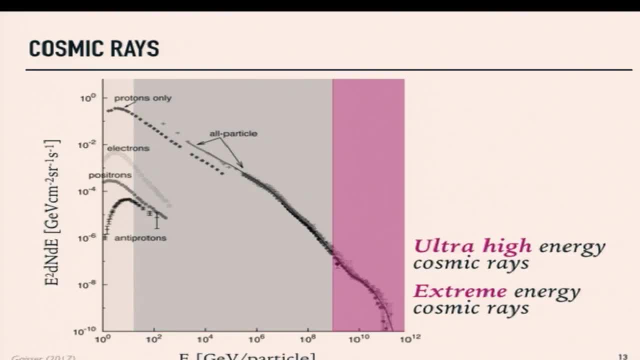 So small spaces being our galaxy here. And that brings me up to the ultra high energy and even extreme energy cosmic rays. These are kind of a subset of the ultra high energy cosmic rays, And then what we really see here is there's actually quite a dramatic cutoff in the spectrum. 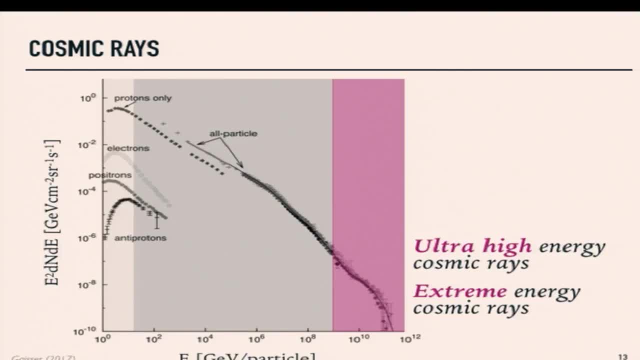 It doesn't keep going with this kind of straight line power law, And this is good, because now we've run out of adjectives to describe the energy of these particles, And these particles are really where I'm going to be spending the rest of the talk. 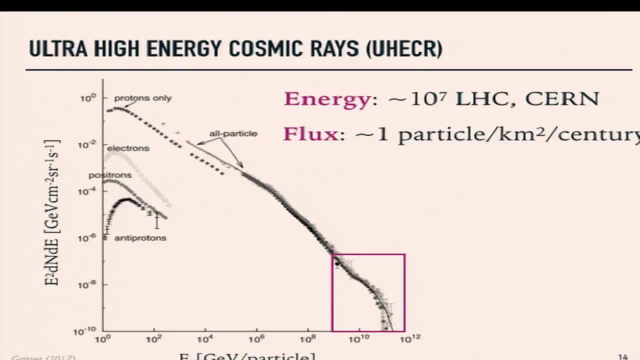 So I'm going to pause a moment and kind of try and get a feeling for what kind of physics we're dealing with here, And so I've tried to convert the scale of this plot into something more familiar. These particles are really high energy. 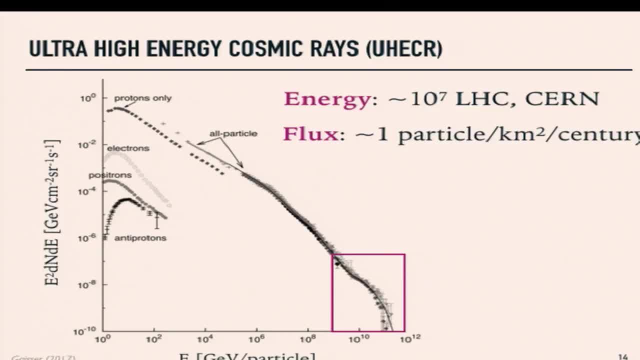 hence the name, And it's kind of hard to connect and convey what this means. So the definition of ultra high energy is particles with energy above one exa electron volts. This is one times 10 to the 18 electron volts And a very common analogy people like to use here. 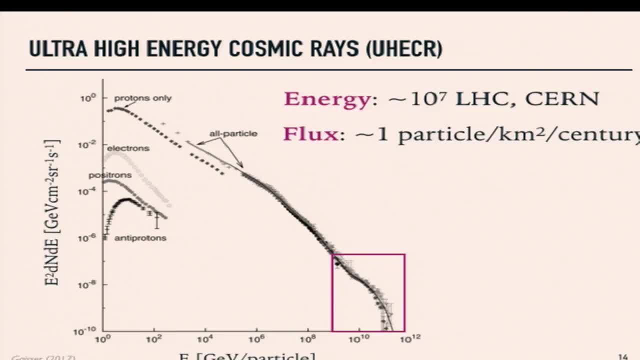 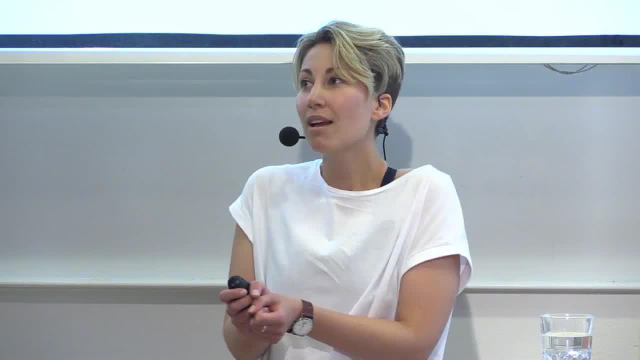 is that's the same amount of energy in a very fast-moving tennis ball that's just been served, but compacted into a tiny, tiny single particle like a proton, And I think this is a good, accurate analogy, but sometimes I feel that it leads me. 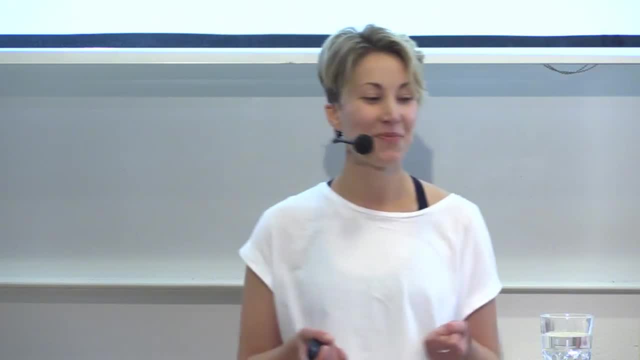 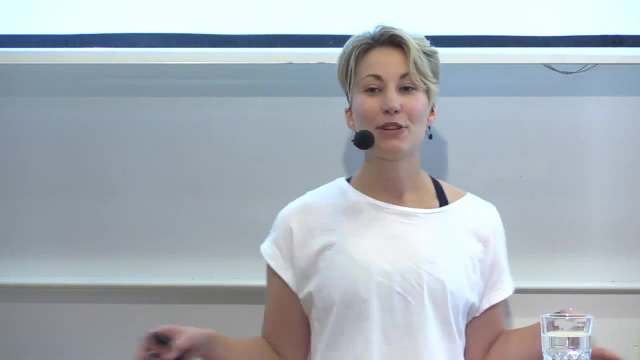 to lose some of the coolness. I mean a tennis ball is not super exciting. So my favorite way to explain this is that at the Large Hadron Collider in CERN, which I think everyone knows is kind of a very high energy experiment, 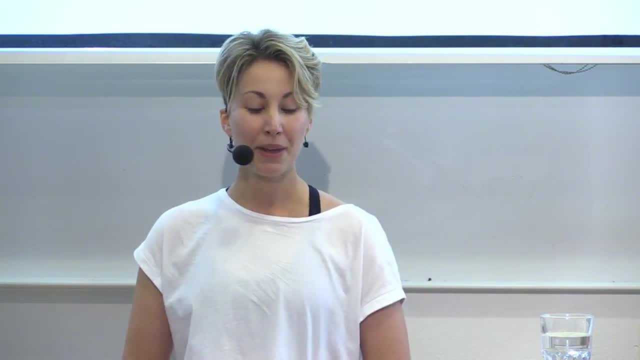 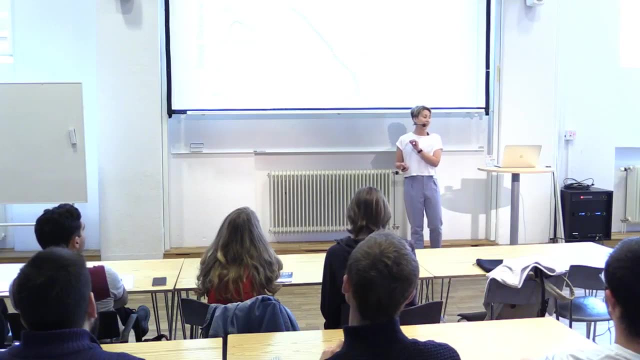 It's kind of one of the best known experiments in high energy physics. I'd say The center of mass energy for two colliding protons is about 12 tera electron volts, So the energy we're looking at here is actually 10 million times higher than that. 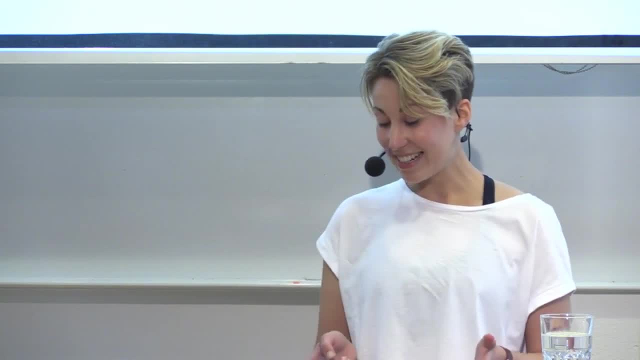 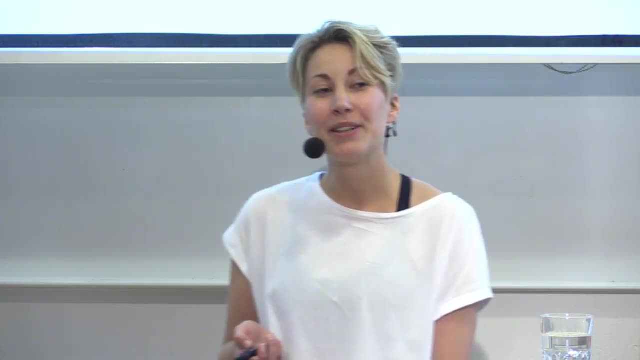 So that's pretty exciting And kind of. secondly, the flux of these particles is extremely low. So if you But it hits one particle per square kilometer per century, So you can probably imagine it's very difficult to even try and think about. 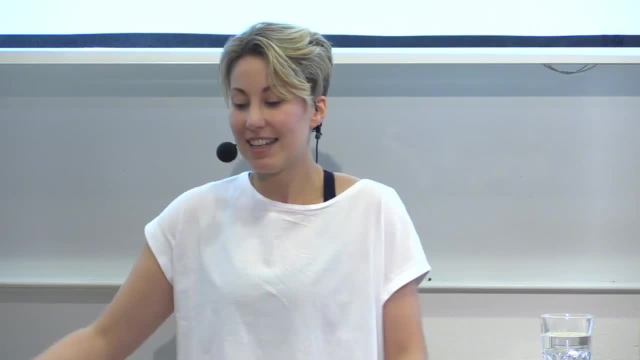 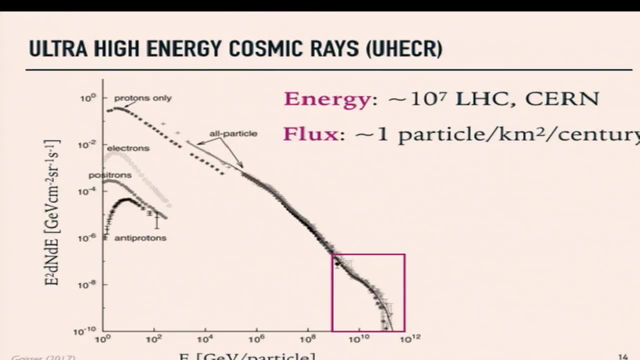 how to detect these particles. I mean, if you have a kilometer-square detector, you're going to have to wait a century to see one. But, as you can see, we have data points so we are able to detect these particles. 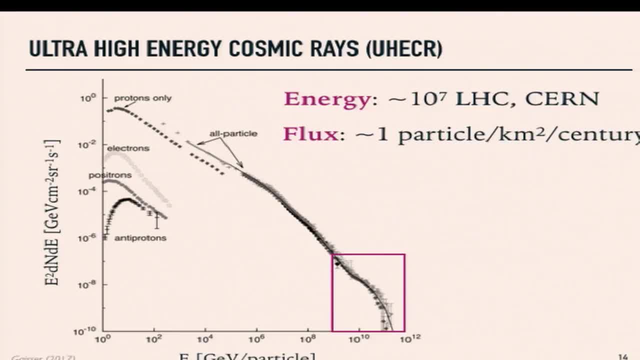 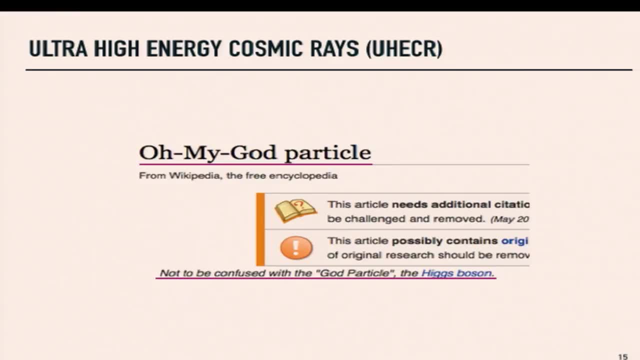 That's something I'll come back to later in the talk And actually one of the first detected extreme energy- cosmic rays- has its own Wikipedia page. It's that exciting And kind of in analogy with the results of Hess- the unexpected way that he saw this big increase of radiation. 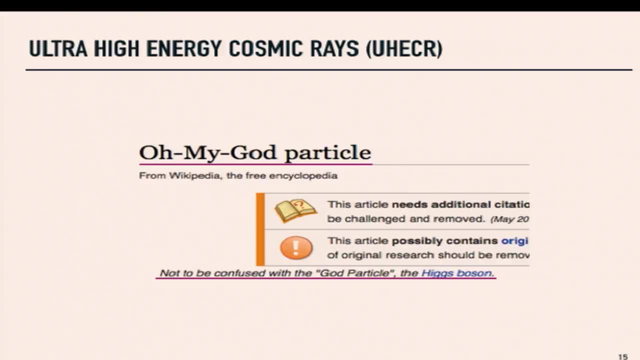 the detection of the oh-my-God particle was quite shocking Because this was in 1991, and at that time many scientists believed that it wouldn't actually be possible to detect these particles at such extreme energies, or that they would even exist with such extreme energies. 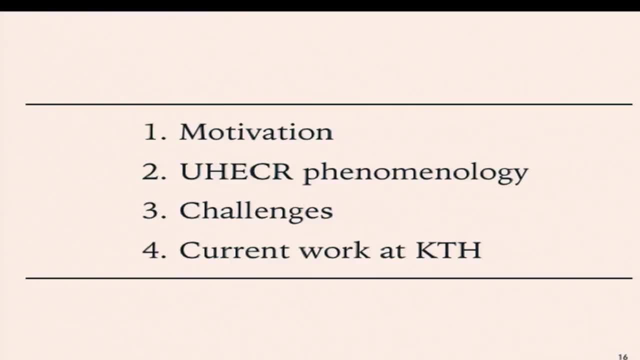 So that kind of wraps up the first chunk of my talk. I'm going to spend the rest of the time talking about these topics in more detail in the framework of the ultra-high energy cosmic rays. So I'm going to start with the motivation. 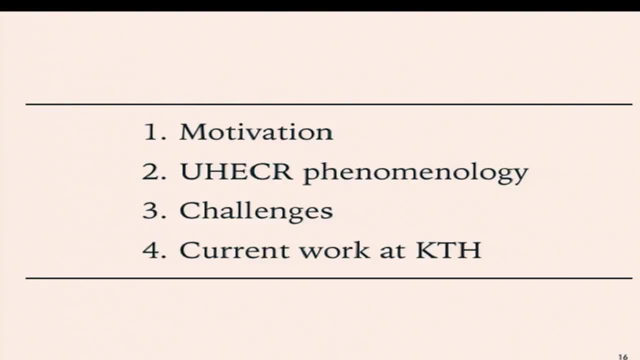 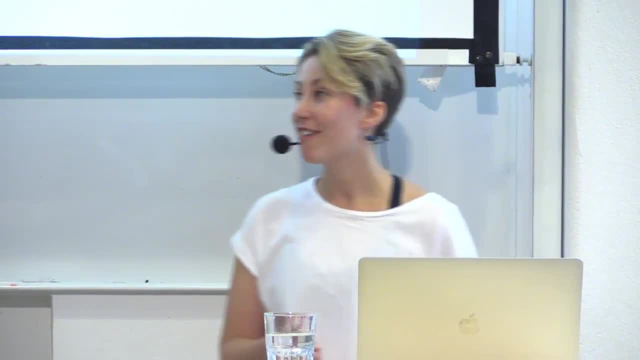 like: why is it interesting for us to study this, other than it's cooler than CERN, obviously? Then I'm going to talk about what I've called ultra-high energy cosmic ray. That's what this acronym means, by the way, If you write it out all the time. 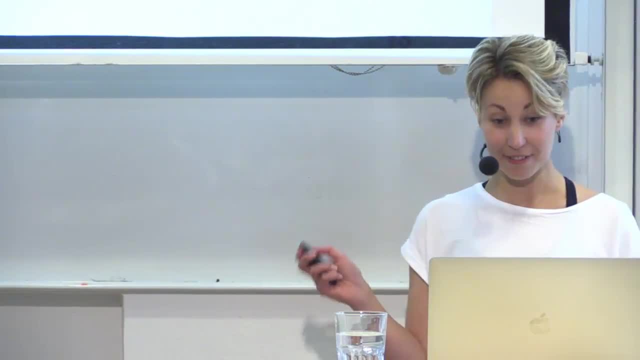 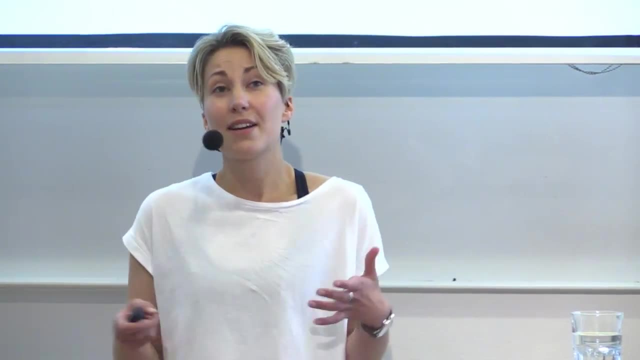 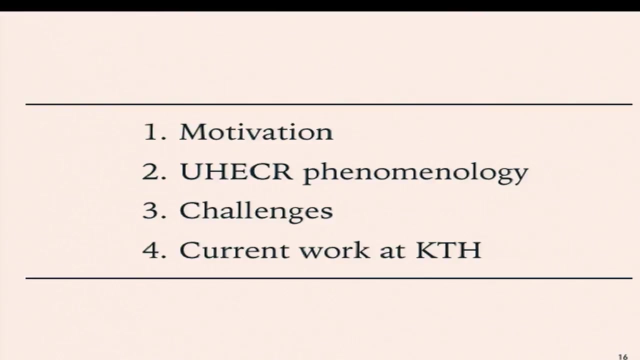 your slides are just full of the same words. So ultra-energy cosmic ray phenomenology- What I mean by this is just the kind of what we think we know about ultra-high energy cosmic rays and the working hypothesis of the research area and the theories that we're basing our current work on. 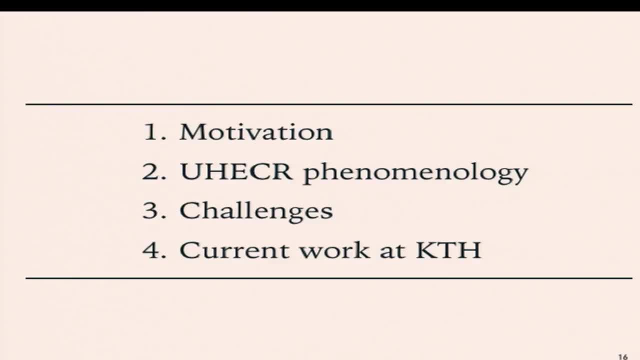 Then I'm going to talk more about the challenges, so what we don't know, and then connect back to what is happening at KTH right now in order to challenge those challenges, And this is probably what I'm supposed to talk about. so I'll finish there. 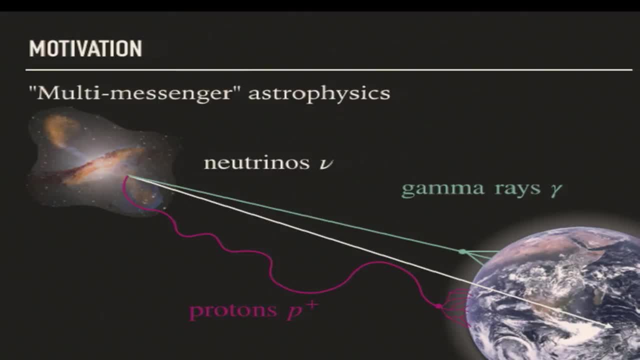 So I'm going to start with motivation, So zooming out a bit what is really the bigger picture here? Connecting back with the title of my talk, I said exploring the universe. So that rather grandiose, grandiose statement really means. 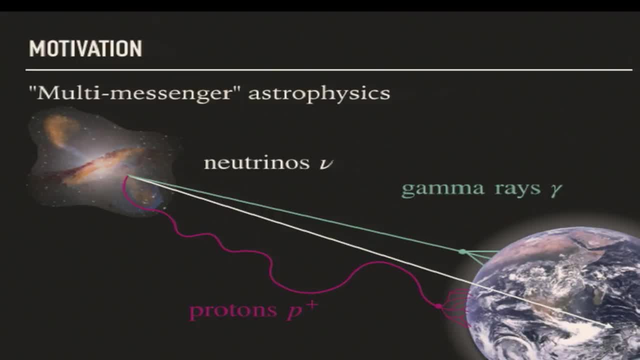 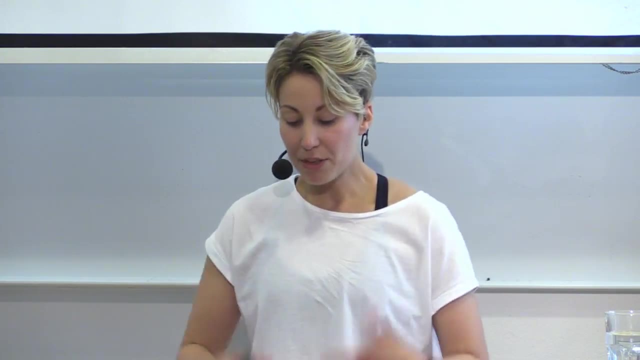 we want to know more about what's going on out there And, as I said, the ultra-high energy cosmic rays are believed to be extra-galactic. so from outside our own galaxy, And also in order to be the extremely high energies that they are, 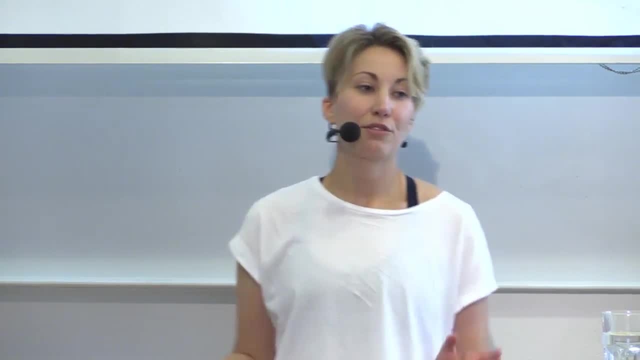 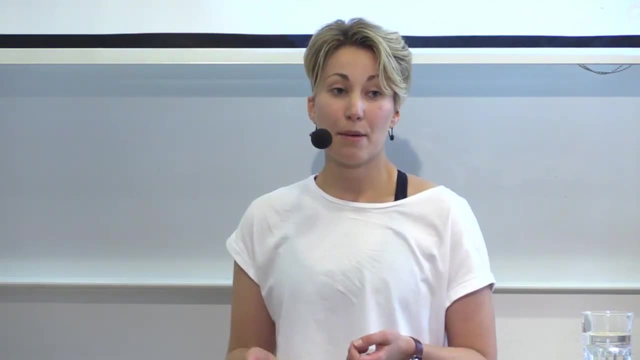 they must be produced in some kind of very dramatic, violent astrophysical event that's capable of accelerating them. And if we want to learn more about these events, perhaps one of the most obvious things to do is look at them with light, with a telescope. 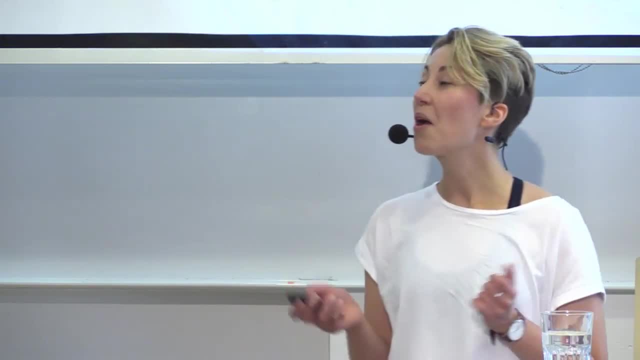 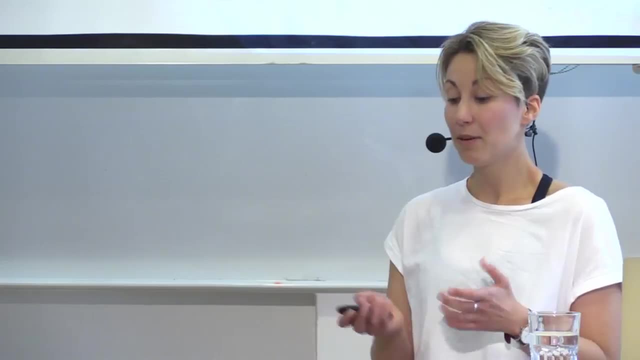 And indeed that's what people have done for centuries. And if it's something- very high energy, you might think, okay, let's look at higher energy light like gamma rays, And this is indeed one way to do it. But what's really fascinating, I think 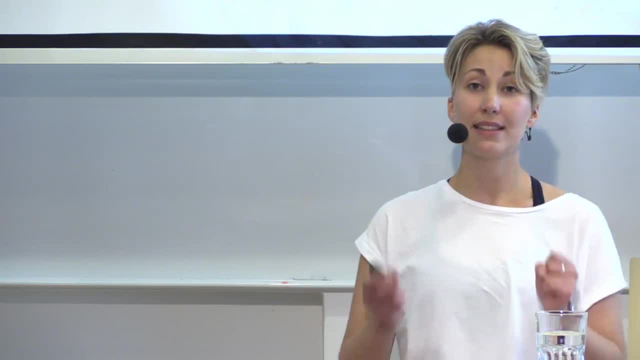 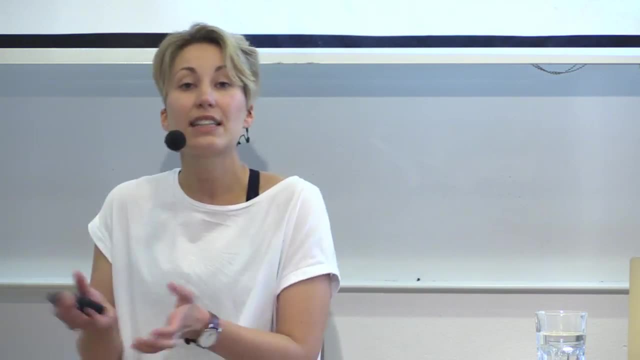 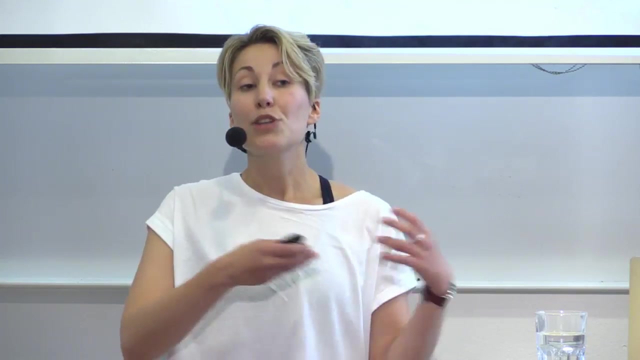 is that it's also possible to detect matter from these distant astrophysical events And, in the same way that photons carry information on what's happening, the physics of these sources, matter like protons and ultra-high energy cosmic rays, can also bring interesting information. 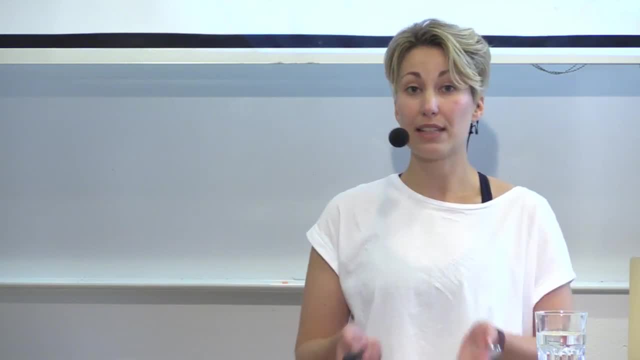 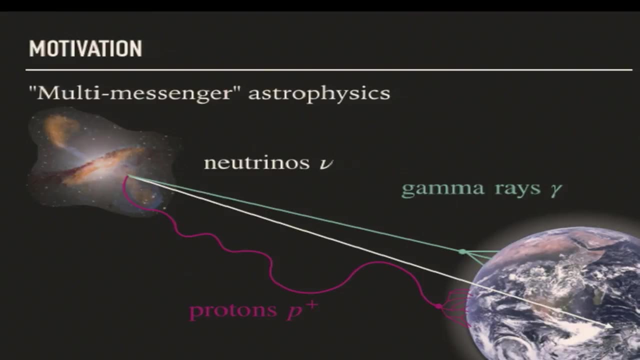 and complementary information on the physics of these sources. So I've tried to summarise that here, this very sophisticated picture, And what's also great to remember is that it is really complementary because things like gamma rays- so this is high energy electromagnetic radiation. 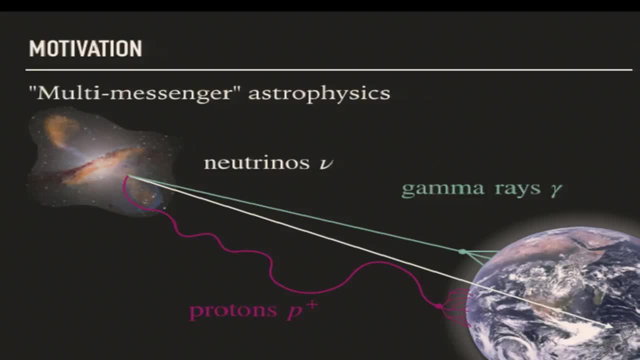 and neutrinos, which are massive particles with very little mass but they're not charged, travel in straight lines from their sources. So this makes them great for doing astronomy, because you can just look at what direction they came from and be like, okay, the source is over there. 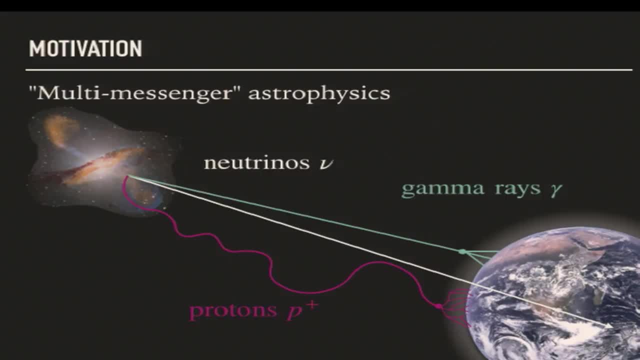 Like we know where it is, So that's good for localisation. Gamma rays can be absorbed on the way towards us, So we might not always see gamma rays, But neutrinos are very weakly interacting, which means that we're almost always. 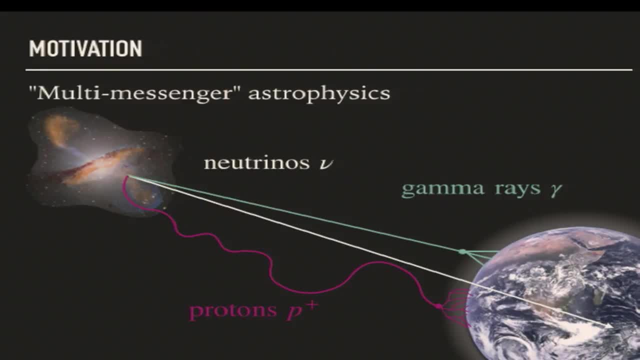 they're always going to reach us, but the problem is because they're weakly interacting. they're very hard to detect. So, as you can see, protons have this kind of funny wiggly path towards us, and this is because charged particles. 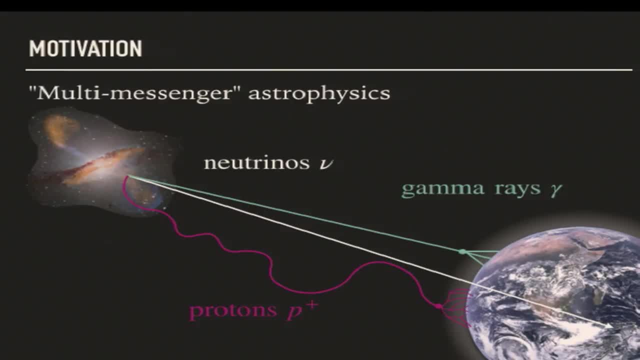 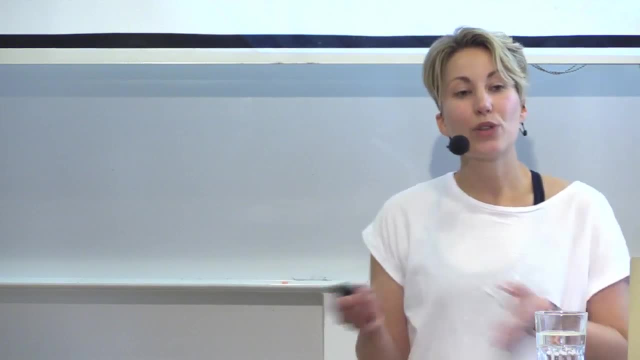 are deflected in magnetic fields. So as we get to higher and higher energies we expect the particles to be much less deflected, but they're still not going to come from exactly where they were emitted, So that makes it a little bit harder. 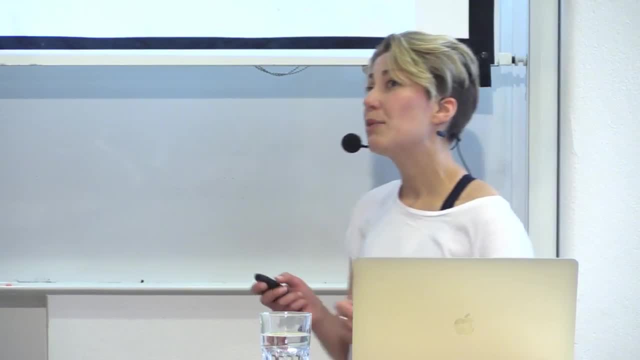 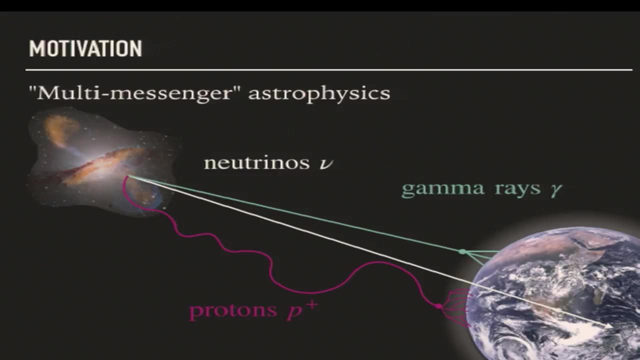 to figure out where they're coming from. But interestingly, we can also use this to infer information on the medium that these particles are travelling through, So they can actually inform us on these mysterious extragalactic magnetic fields and also the magnetic fields in our own galaxy. 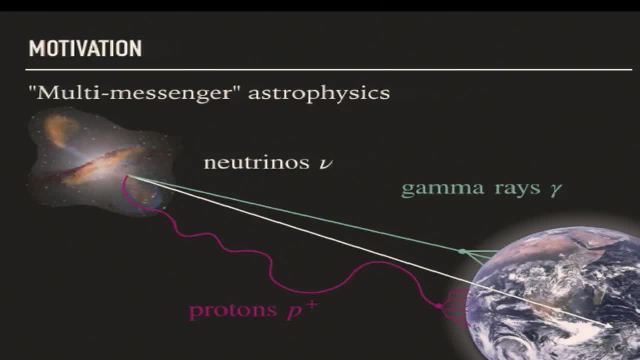 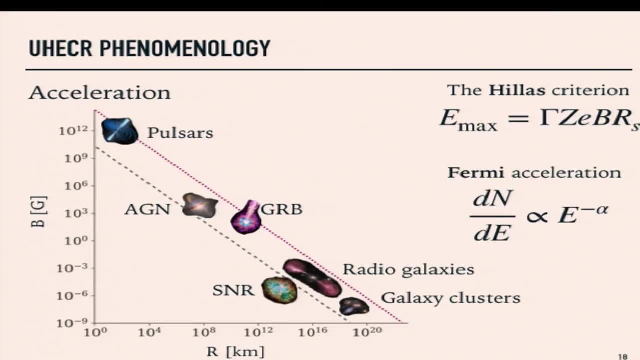 So both the physics of the source and kind of the medium between us and the source, which are things we don't really know about. So now I'm going to talk about the phenomenology. I'm going to do this in a kind of life. 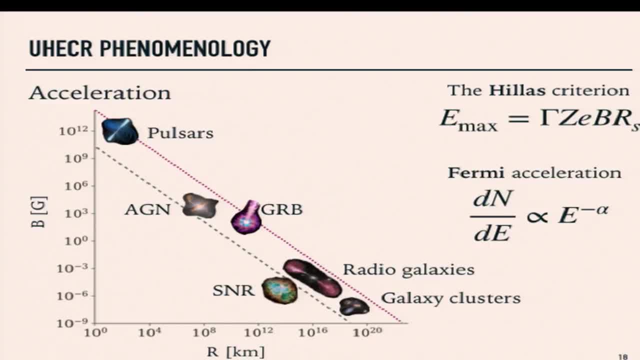 of an ultra-high-energy cosmic ray story. So we're going to start at the source and the acceleration process. So how? I think probably one of the most interesting questions and obvious questions is: how do we get particles to such high energies? This is not obvious. 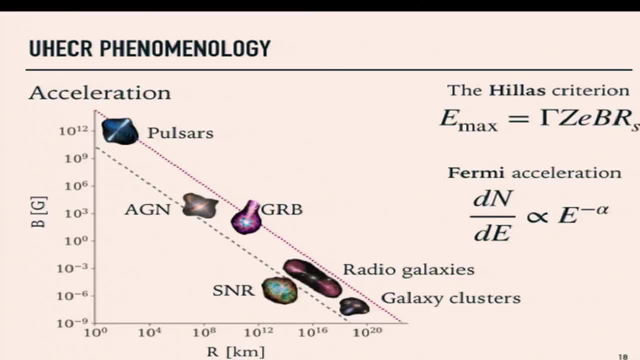 And kind of one of the simplest ways to answer or constrain. that question was put forward by Anthony Hillas, So we have now the famous Hillas criterion in the field, And what he basically said was that if you want to accelerate something, you have to be able to confine it in the source. I mean, if it's no longer in a place where it can be accelerated, it's not going to be accelerated anymore. So his criterion basically states that the maximum energy that can be reached by an astrophysical source is proportional. It's basically the point. 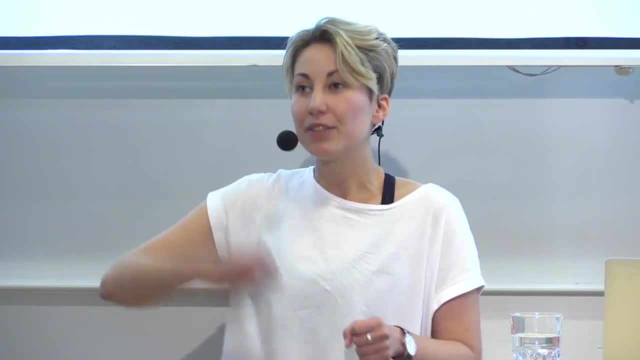 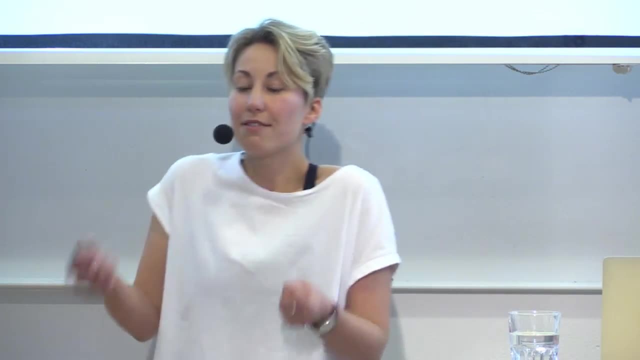 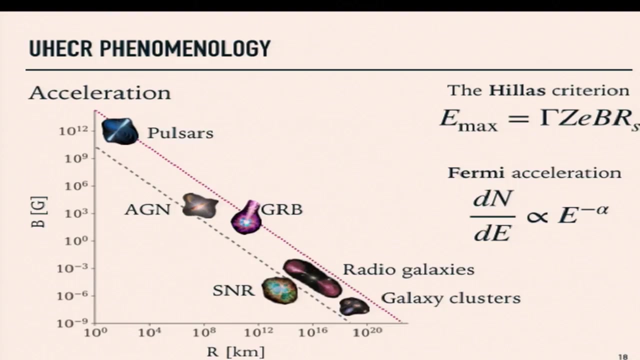 at which the Larmor radius of a particle gyrating in a magnetic field becomes larger than the radius of the source itself, So it can no longer be confined by the most simple magnetic arguments, And so that leads to this statement: where you have the maximum energy, basically proportional. 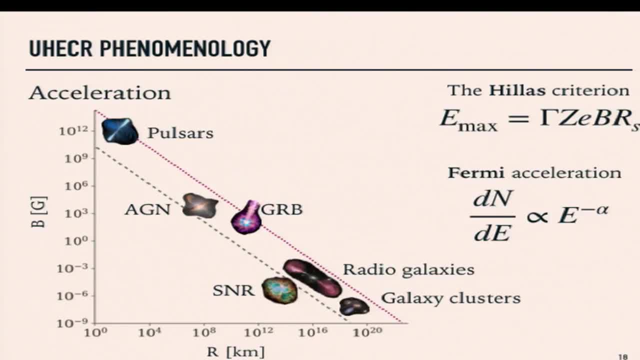 to the charge of the particle, So it's easier to accelerate charged particles, And also to the strength of the magnetic field and the radius of the source. And so that's what I've kind of laid out in this diagram here, And you can plot kind of two extreme constraints. 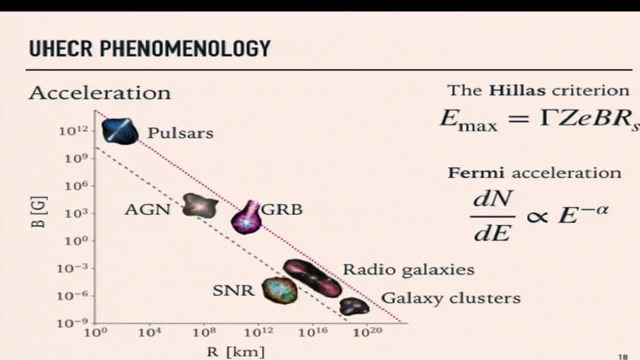 So the pink line is in order to get protons, which are the hardest to accelerate because of their lower charge, to 10, to the 21 electron volts. That's kind of the most extreme case. And then the gray line is to get iron. 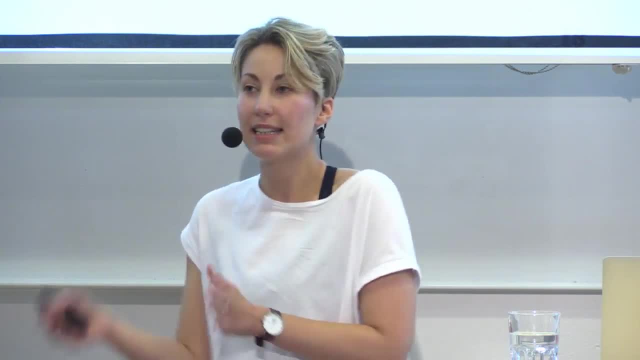 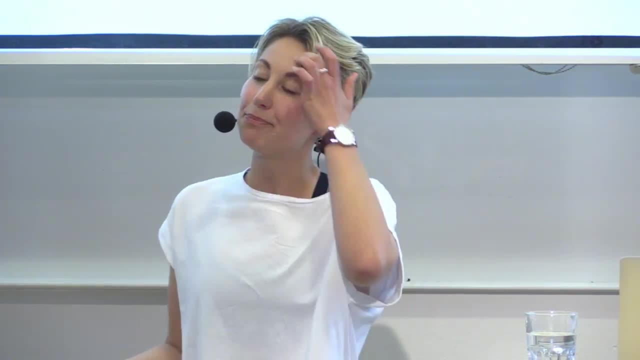 which is much more charged to 10, to the 20s. This is kind of the region of the parameter space that we want to look in if we're going to find what might be accelerating them, And so on this I've plotted some sources. 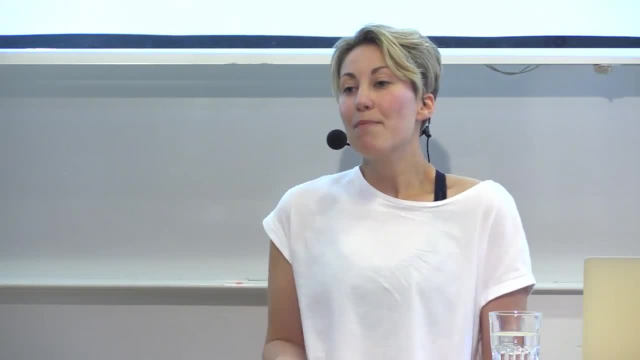 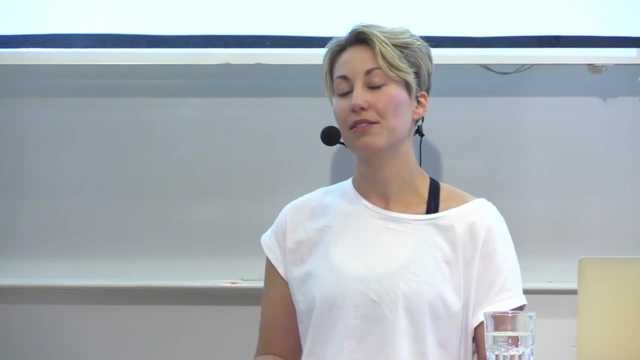 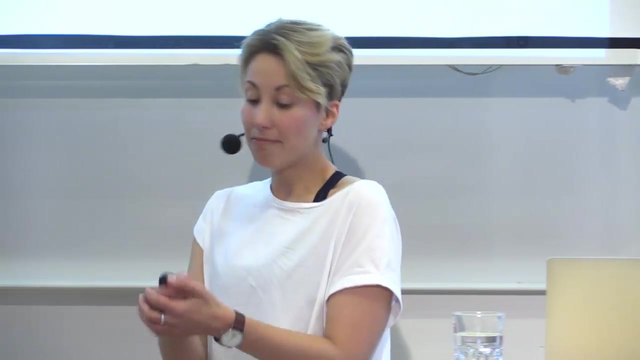 that were present in probably the first Hill-Ass diagram that show very much the kind of popular idea of what are the sources of ultra-high-energy cosmic rays today. So you basically have a kind of trade-off between very small magnetized sources like pulsars. 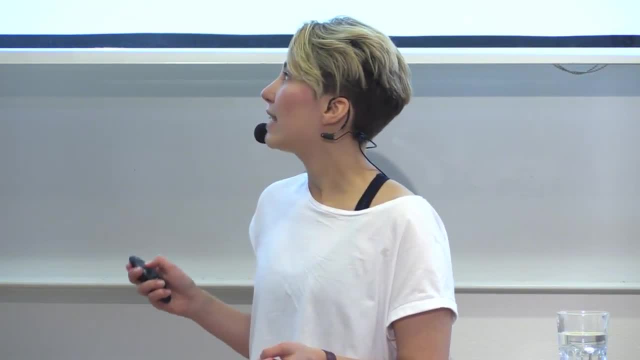 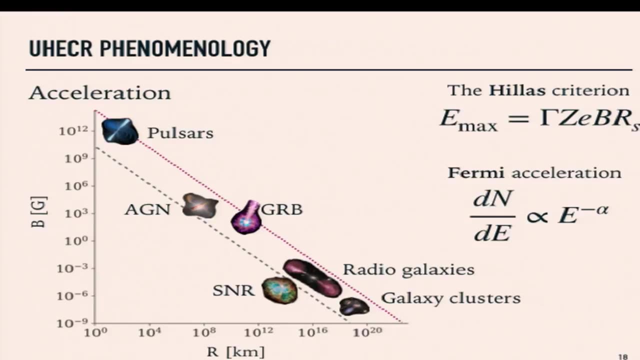 or then coming down in the middle, things like active galactic nuclei, So that's supermassive black holes at the center of galaxies that are creating matter, Gamma-ray bursts, which are kind of two neutron stars colliding, or also thought to be. 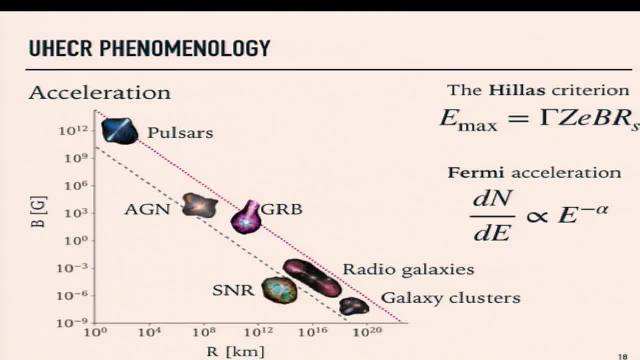 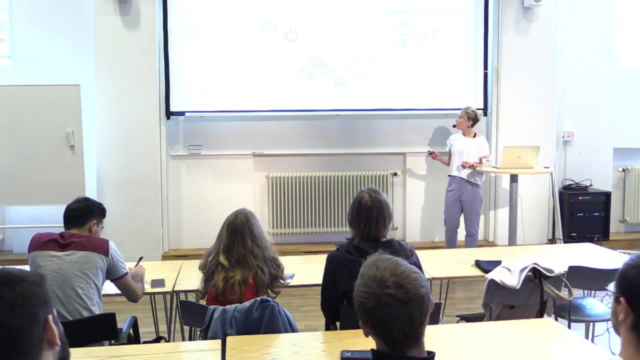 a kind of core collapse, supernova. So these are kind of big, explosive things. And then down here we have kind of much larger scale and less magnetized accelerators like supernova, remnants or galaxies that are bright in radio waves, or indeed galactic halos and galactic clusters. 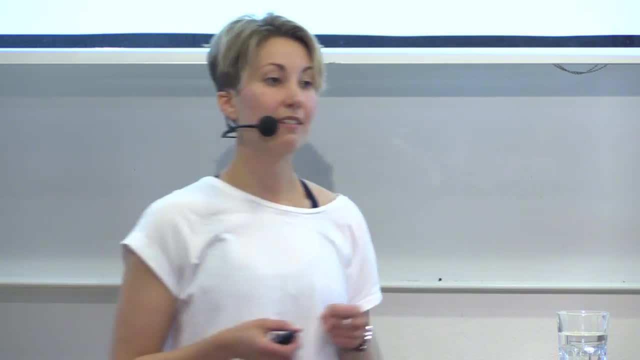 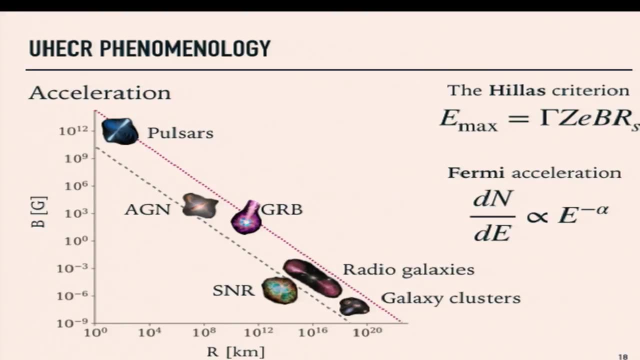 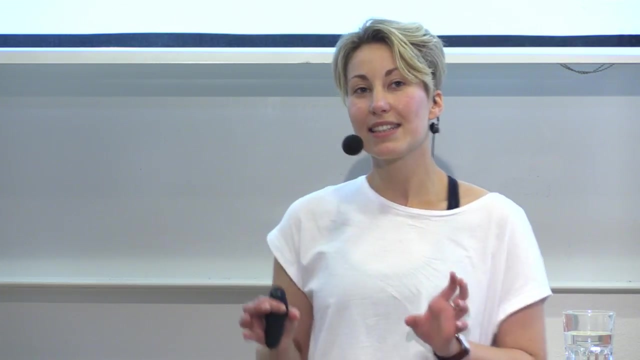 And so, whilst this is very much still an active research area and we don't really know exactly how these particles get to such high energy, the working hypothesis is that we have Fermi acceleration going on And this has two different kind of subsets or different types of Fermi acceleration. 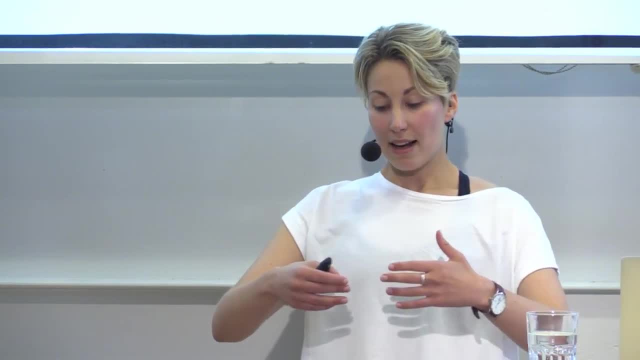 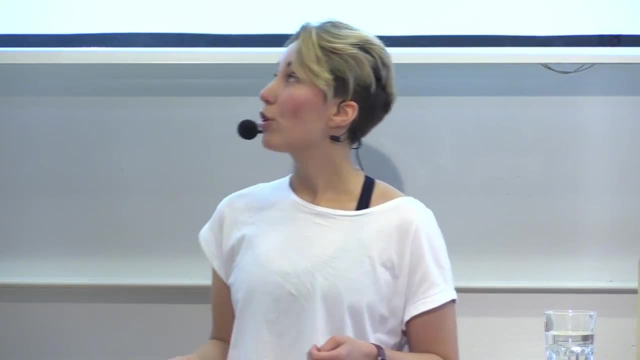 called Type I, which is basically acceleration of particles in astrophysical shocks. So if you have a big explosion, particles can get accelerated as they cross the shock boundary. And then also Type II, which is kind of this larger scale acceleration of particles. 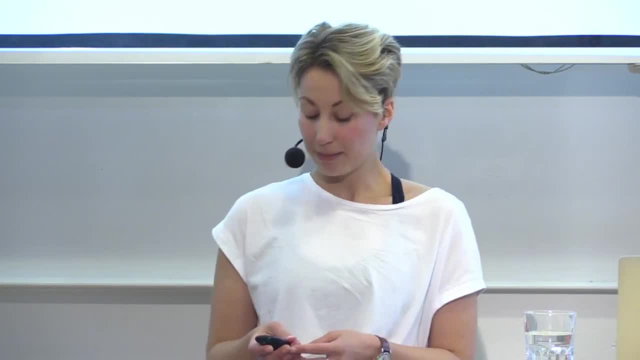 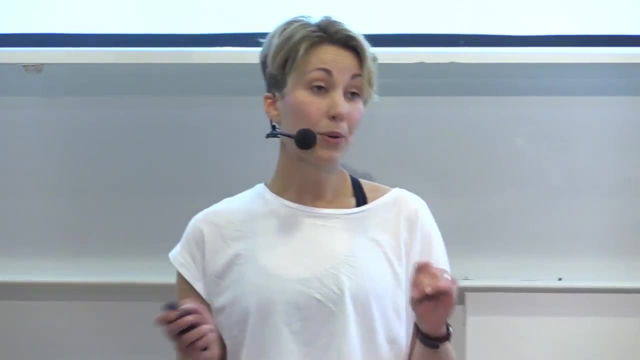 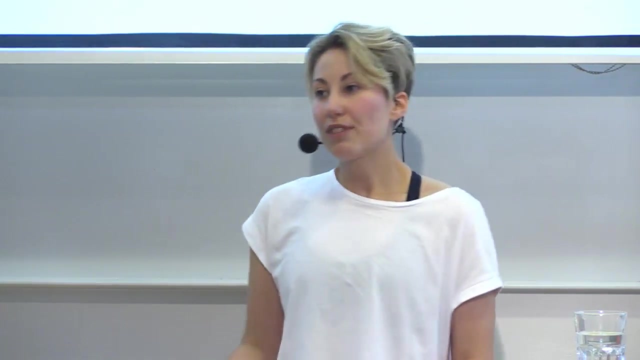 in big magnetic clouds by turbulent processes. And what's interesting is, both of these processes result in kind of the same power law spectrum, which is what I showed back at the beginning, this straight line power law spectrum of cosmic rays, And I think this is one of the reasons. 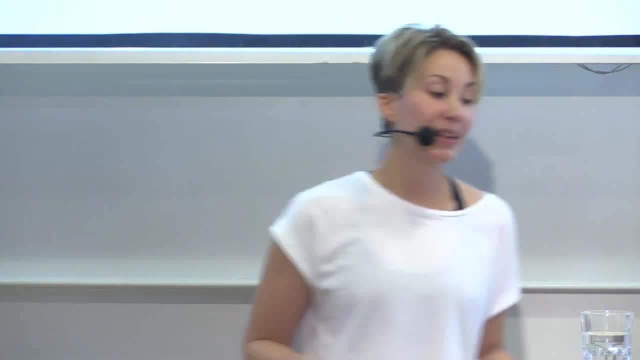 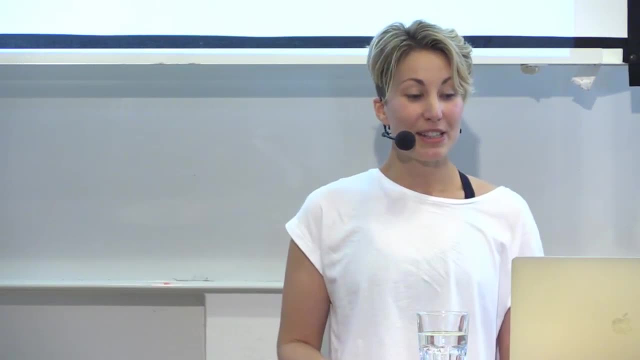 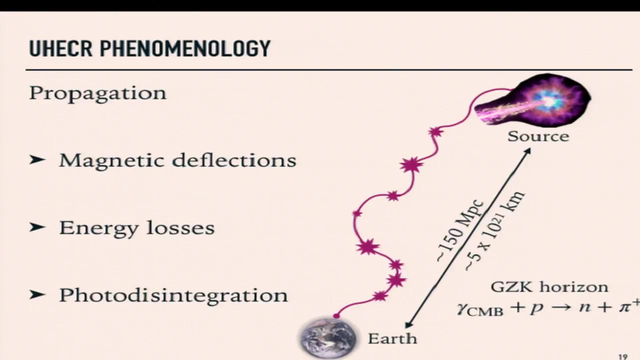 why this has for a long time been a popular mechanism because of this connection. So once we've got some high energy particles, we still have to get them from the source to Earth, And this kind of opens up a whole new load of complexity and different physics. 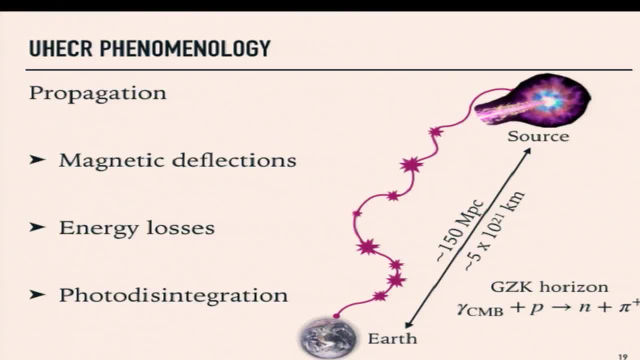 So, as these particles propagate from the source to us, as I've already mentioned, they're going to be deflected by the magnetic fields, And this is going to depend on the strength of the magnetic field, the charge of these particles and their energy. 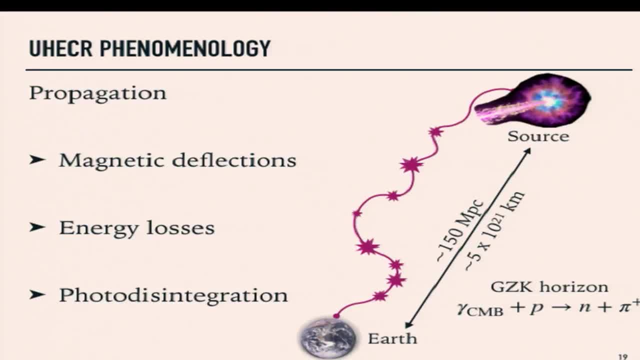 And they're also going to undergo some kind of interactions. It's not going to be a kind of calm, relaxing journey. They're going to have lots of different processes as they travel from the source, the source galaxy, through extragalactic space into Earth. 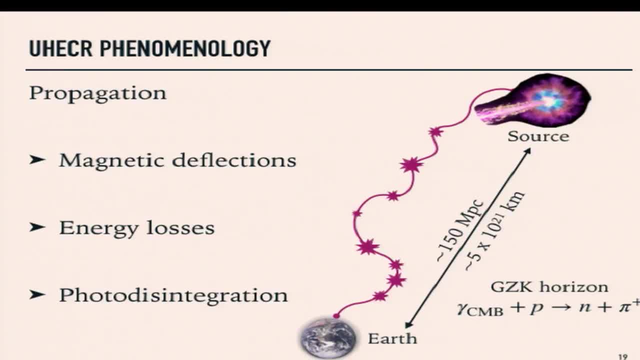 And probably one of the most dominant processes, at least for protons at these energies is because these particles are so highly relativistic. the cosmic microwave background, which is kind of this low-energy radiation that permeates the whole universe, gets blue-shifted. 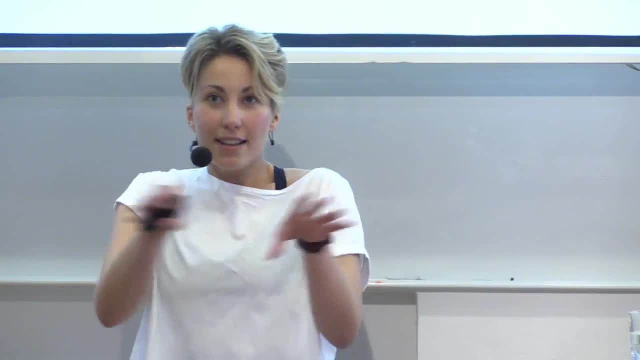 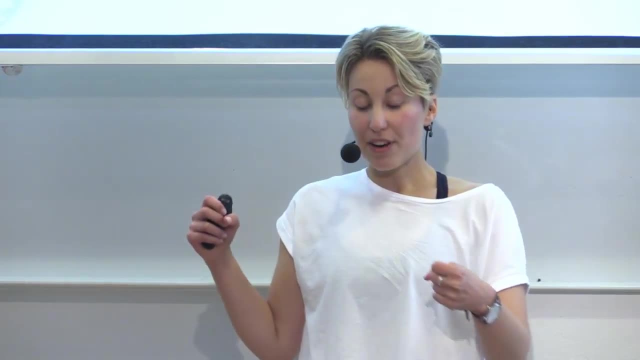 So in the rest frame of a proton it sees a kind of sea of X-rays, of very high-energy radiation, And what this really means is that it becomes very highly probable that this proton is going to interact with that background field and lose energy. 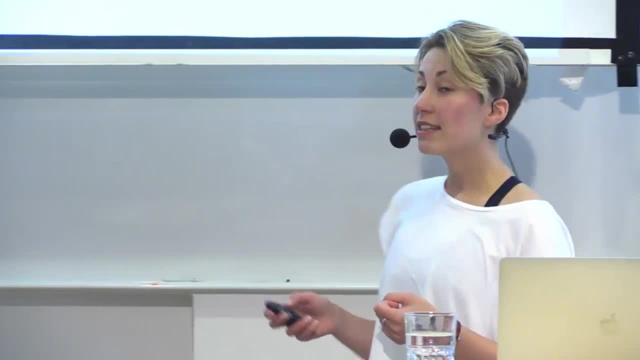 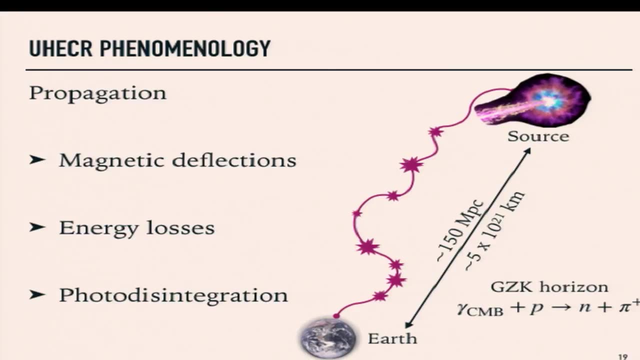 And the first people to propose this were Grison, Zatzepan and Kuzmin. So this is why we have this GZK acronym here, because what they noticed was that you know if we're going to get very ultra-high-energy cosmic rays. 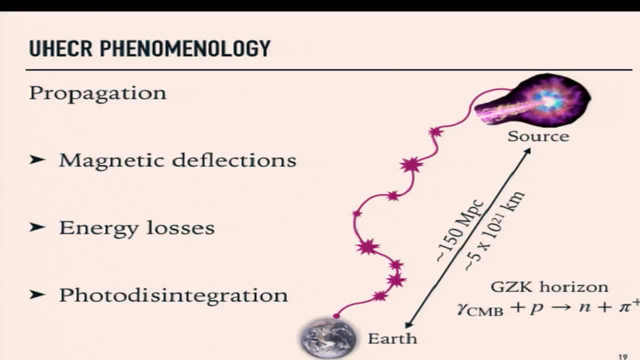 at the Earth. they can't have come from very far away because they would have lost all their energy interacting with the cosmic microwave background. So we have what's known as the GZK horizon and that tells us that the ultra-energy cosmic rays 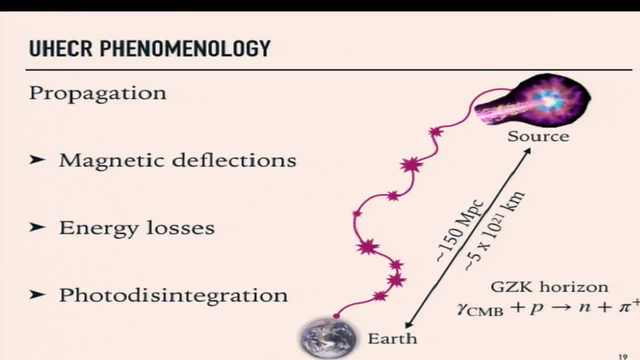 must come from within the nearby universe. So that kind of gives us a clue as to where they might be coming from. And I say nearby universe The kind of typical GZK horizon distance is around 150 megaparsec is kind of the units. 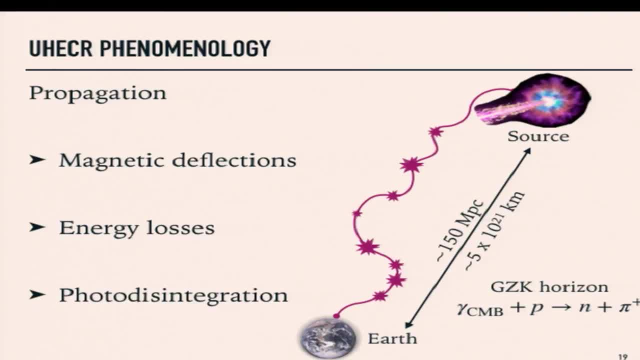 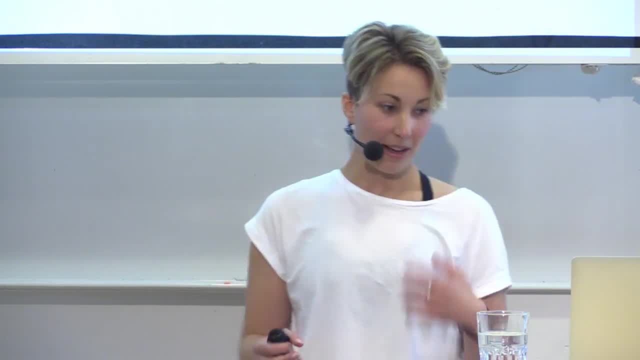 we usually use in the literature And this converts to about 10, to the 21 kilometers, So it's really far. It's definitely well outside of our galaxy and into the nearby universe, but not on the kind of same cosmological scale. 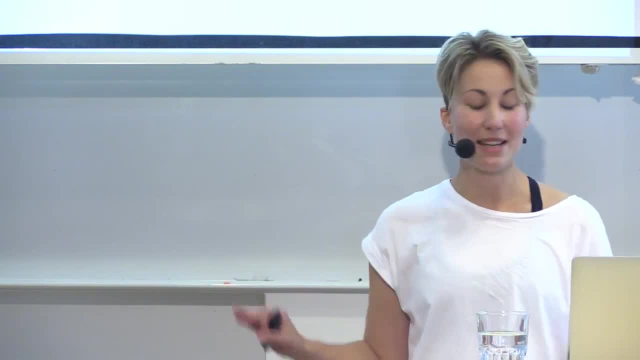 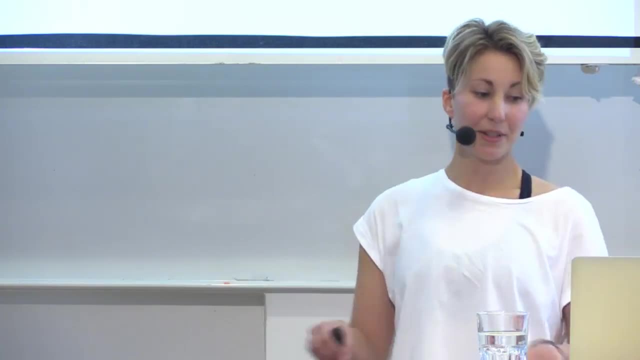 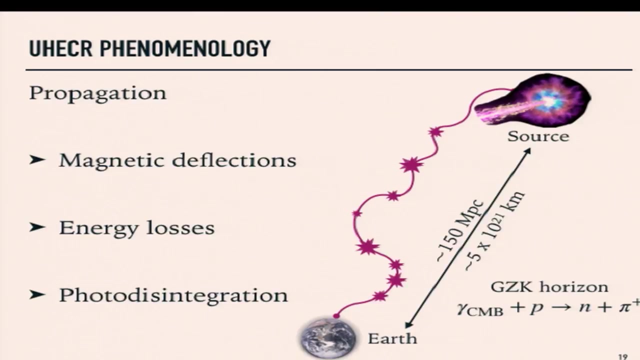 So it's still well below a redshift of one, if that means anything to anyone. So finally, as the cosmic rays propagate, they also- if they're not protons and they're heavier particles- they're going to lose energy and break apart. 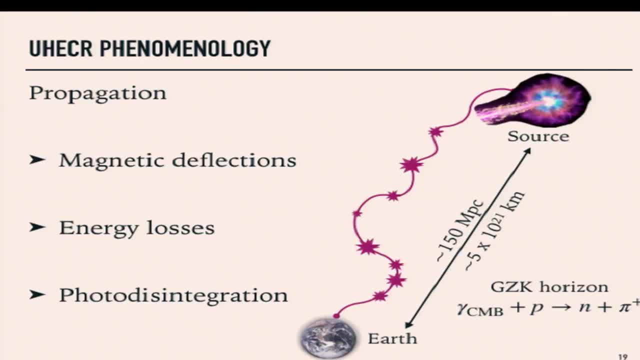 So their type of particle is actually going to change as we propagate from the source to the Earth. So there's really a lot going on, and if we want to figure out what's happening at the source, we have to kind of go backwards. 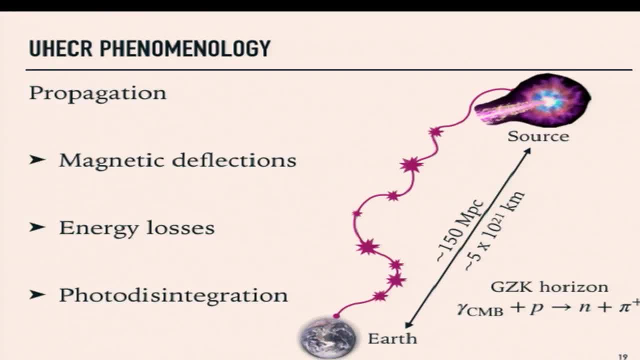 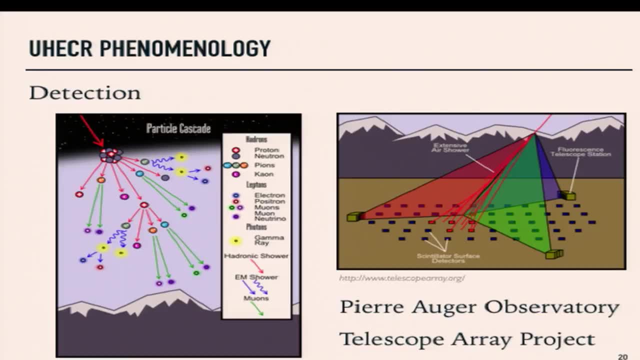 and there's a lot of things that we don't know. So, finally, a cosmic ray arrives at Earth, but it's not over yet. Now we have to figure out how to detect these very rare particles And, as I mentioned before, we've got about. 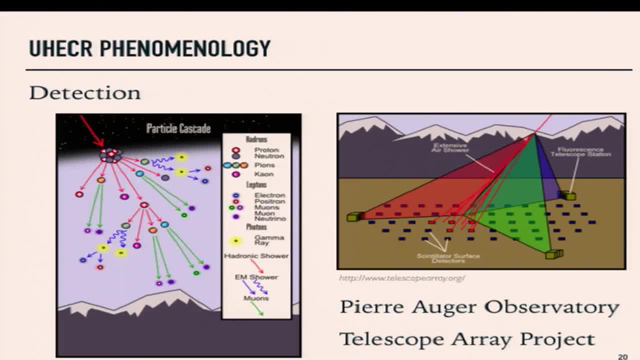 one per square kilometer per century. So what we do is actually use the entire Earth's atmosphere as a giant calorimeter, And we do this by building kind of large arrays of particle detectors on the ground And in combination with these kind of fluorescent rays. 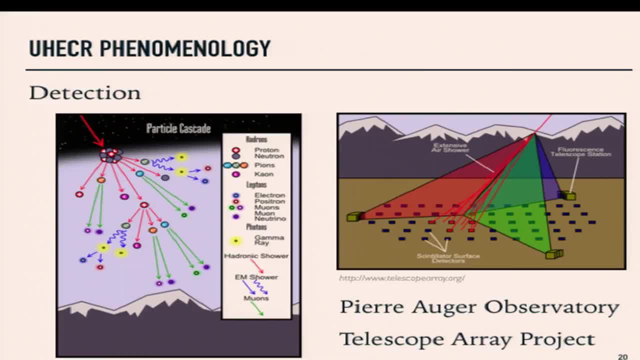 and with these kind of fluorescence telescopes, because what happens when a very high energy particle hits the atmosphere is it creates what's called an extensive air shower, So it's a big particle cascade and the end result of this is the excitation of nitrogen. 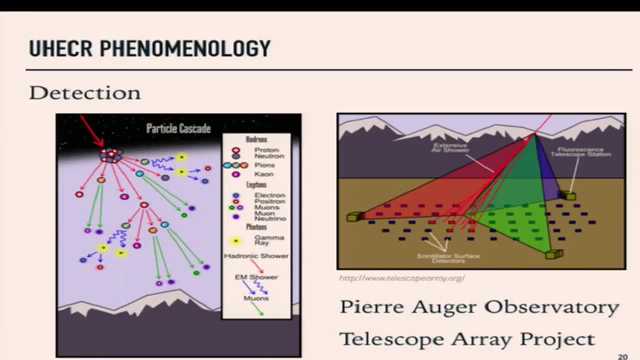 in the atmosphere, which is the most common element, And then this de-excites and produces radiation in the ultraviolet wavelengths, So that can be detected with these kind of fluorescence telescopes. And then we also catch the particle footprint of the shower on the ground. 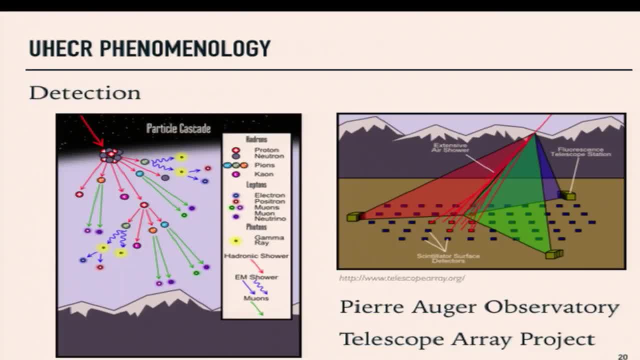 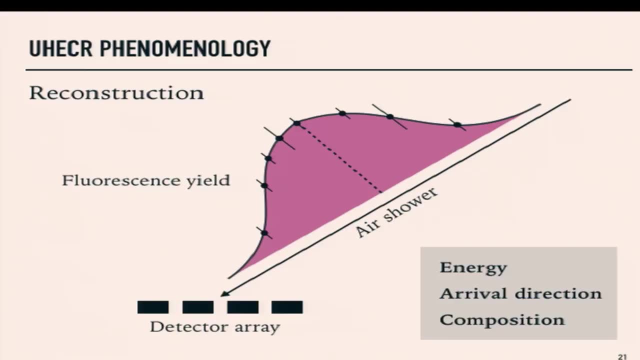 with these particle detectors. There's two observatories doing this, one in the southern hemisphere called Pierre Auger Observatory, and another in the northern hemisphere, So they observe different parts of the sky And from this information we can reconstruct the initial energy. 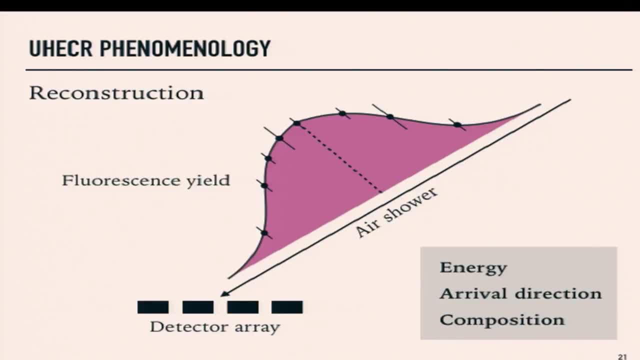 of the particles, which is basically how much stuff is produced in the shower and then also where they come from on the sky. So that's just the direction that the shower is following And then also the type of particle, and this we can do. 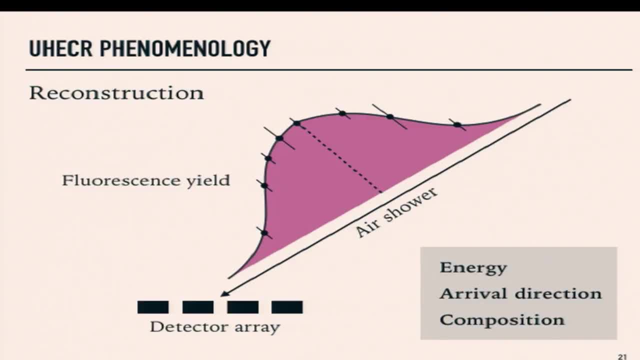 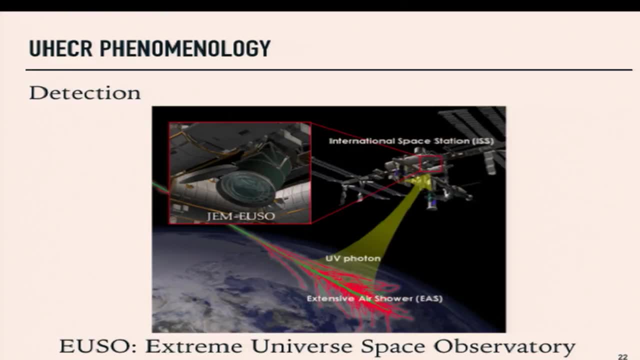 from the shape of the shower, kind of how wide it is and what kind of particles we detect on the ground. So, whilst not yet in existence, one way to do this would be to take the fluorescence detector technology from the ground and put it in space. 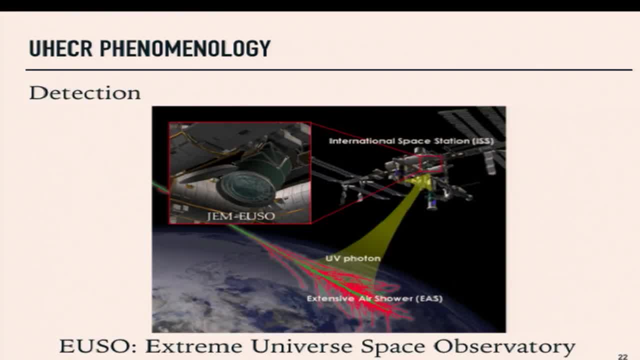 And the motivation for doing this is really to be able to observe a much larger amount of the atmosphere at any one time. So we are capable of detecting these particles, but we still don't have a lot of data, So it would be nice to have more. 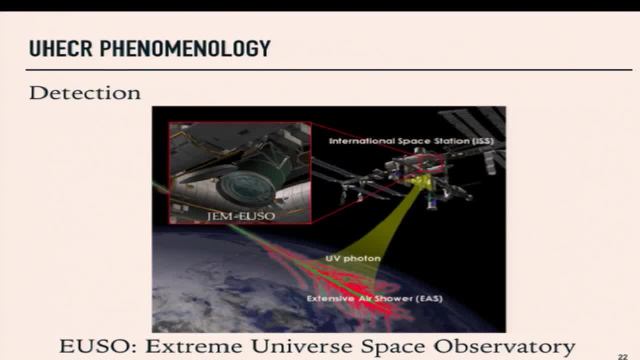 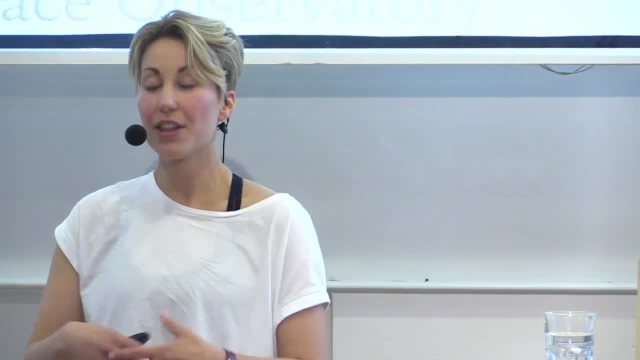 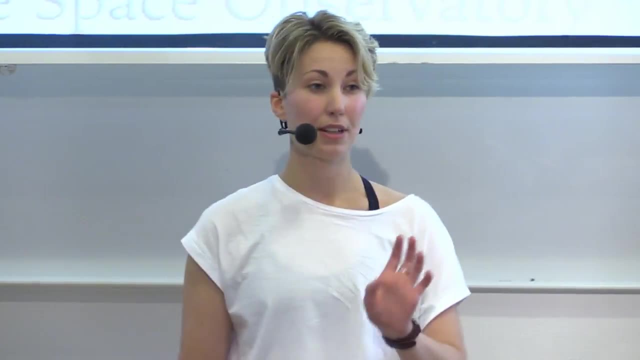 so we can learn more, And so increasing the statistics is one motivation for going to space, And another would be that because right now we can only observe each hemisphere with a different detector and it's really difficult to combine these results and understand the different systematics. 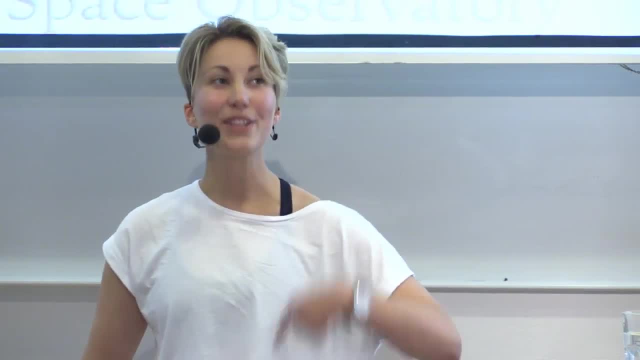 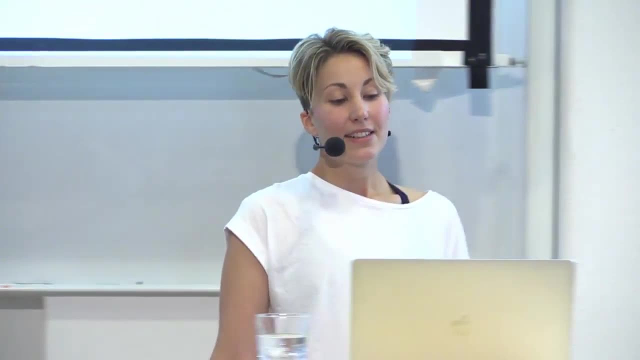 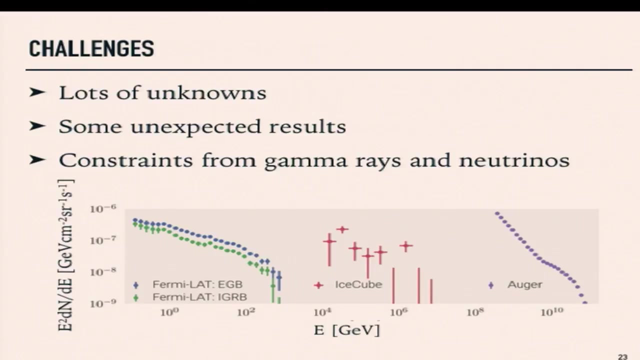 between the two instruments. It would be nice to have one detector that could orbit around the Earth and observe the whole sky, to kind of resolve these conflicts. So I think the challenges have maybe made themselves a little bit evident in that description of the physics behind cosmic rays. 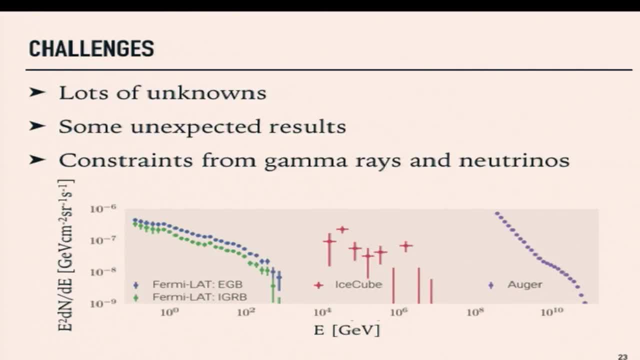 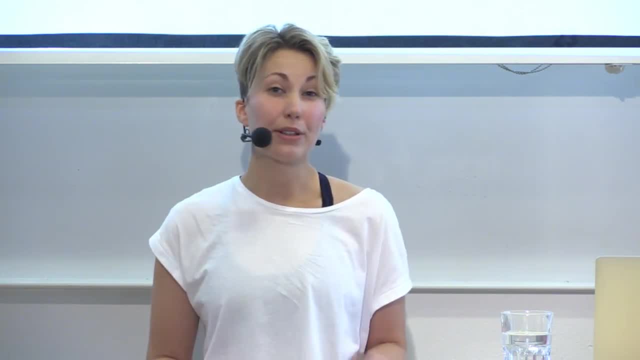 We have a lot of unknowns, some expected results. For example, we now believe that the highest energy particles are actually heavier than we thought. they're probably not protons or some mixture. And finally, coming back to that bigger picture, if we want to be able to explain, 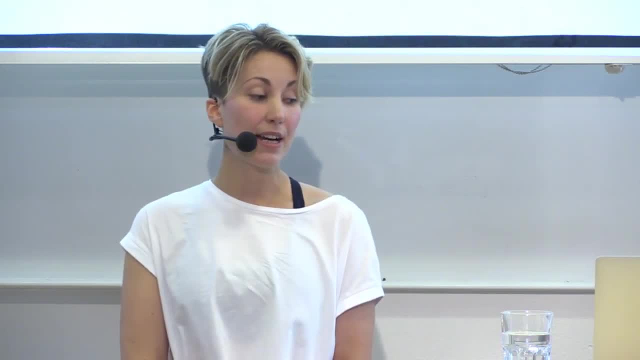 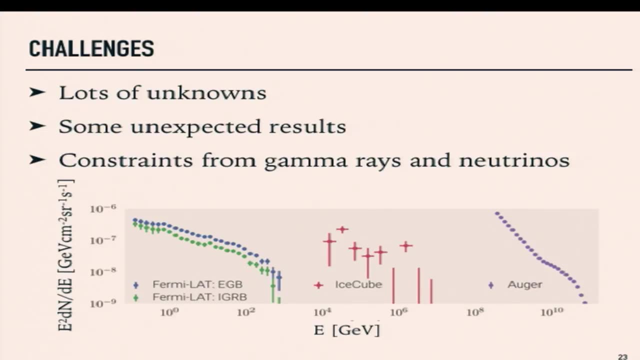 the ultra-high energy cosmic ray spectrum that we see at Earth with some model. so this is the data from the Pierre Auger Observatory. here the energy spectrum we're going to have to be able to be kind of in accordance with the other data. 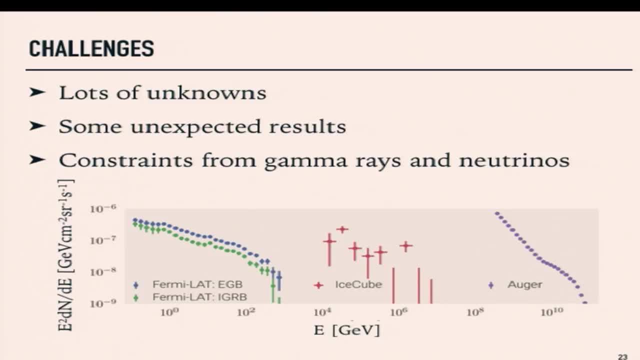 that we have on gamma rays and neutrinos, And so this is the IceCube energy spectrum for neutrinos and here gamma ray data from the Fermi instrument. So if you want to answer one question here, you're going to have to kind of 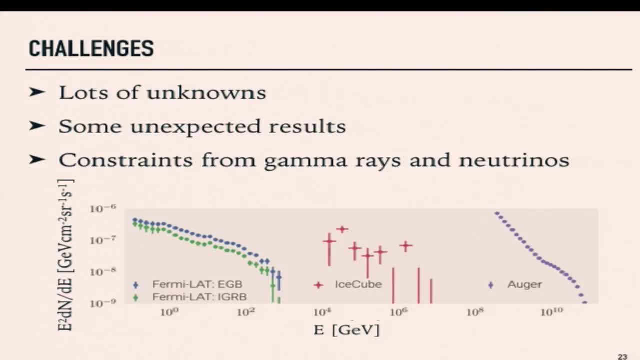 also tackle the others at the same time. So it makes it difficult to come up with crazy models that might produce loads of neutrinos or no gamma rays. There has to be some balance between them. So we have some clues about what's going on. 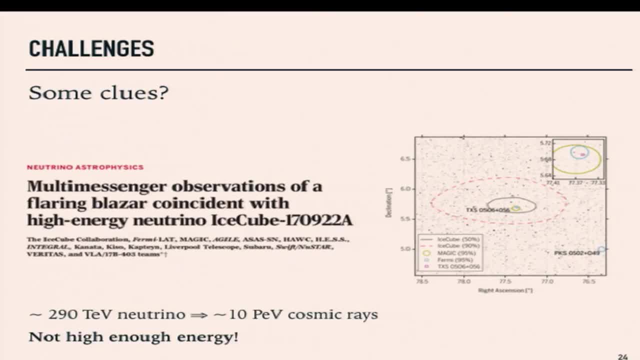 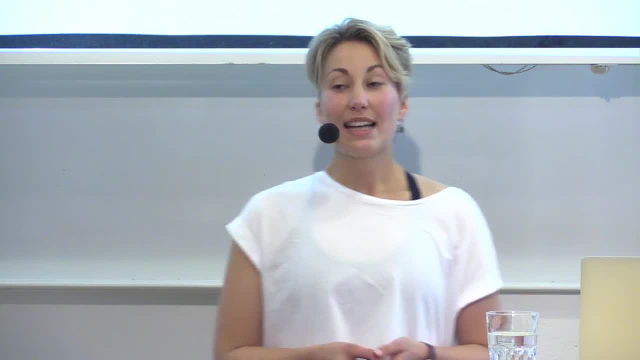 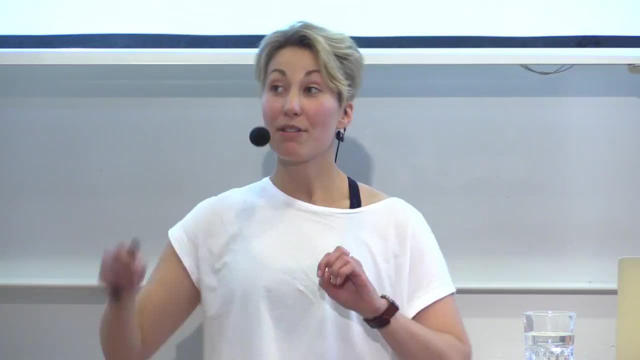 But yeah, I'm going to mention this because it was very recent news that I think might have made it to actual non-science news. There was an announcement by the IceCube collaboration that they detected a neutrino in coincidence with a gamma ray flare. 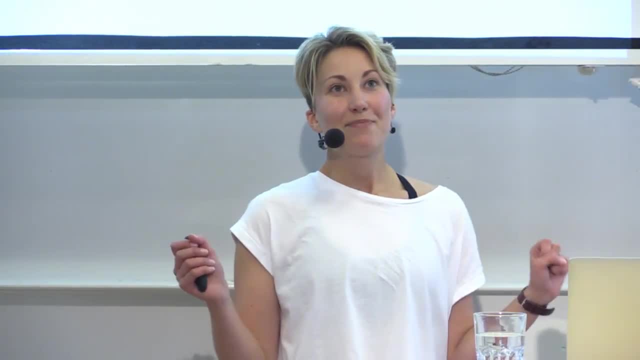 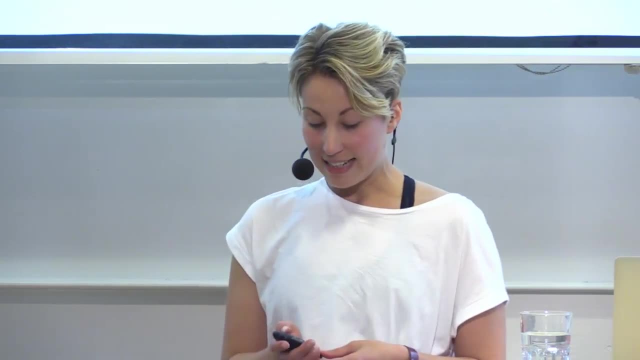 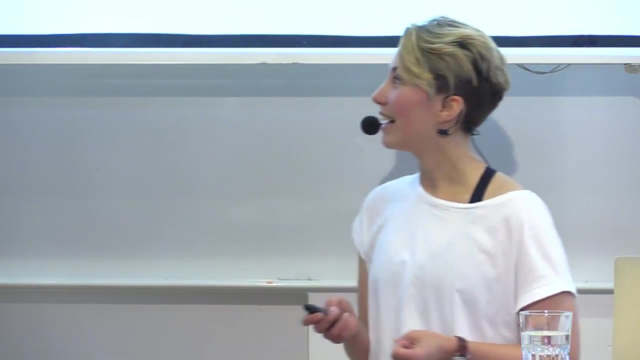 from a blazar. So a blazar is basically a black hole with its jet pointing towards us, so it's very bright in gamma rays And they saw one neutrino which they think came from this source and there's two papers about that. 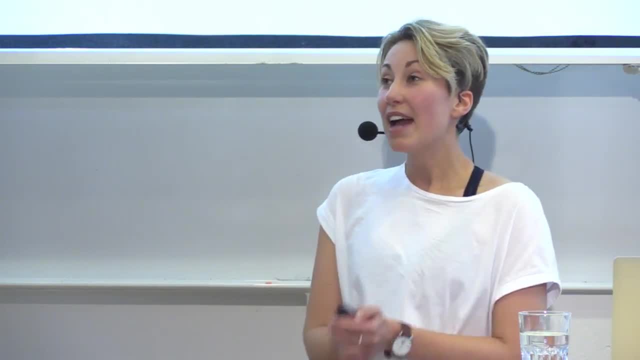 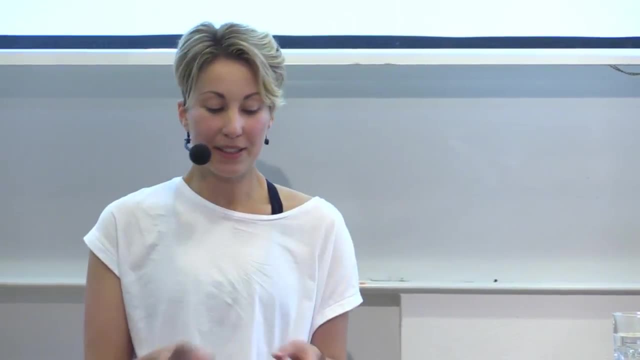 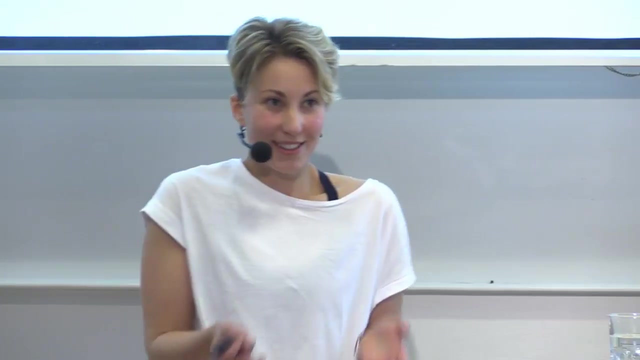 And a lot of people are then thinking: okay, well, this is really kind of a sign that we have ultra-energy cosmic rays produced here, because the processes and the physics which accelerates protons or particles is also going to produce neutrinos and gamma rays. 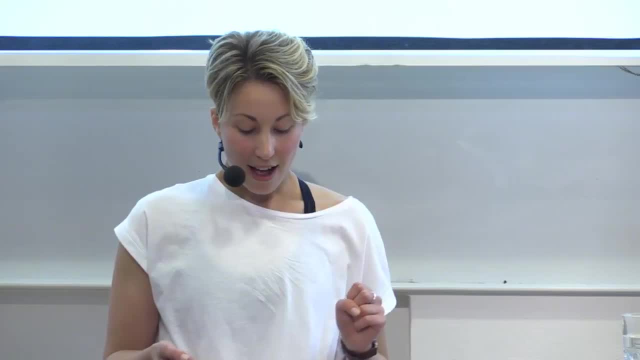 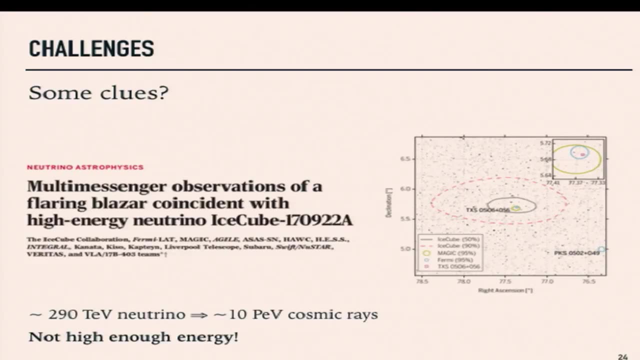 This is one way to kind of get at the sources, But looking a little closer we see the kind of energy neutrino that they detected. it gives us about a 10 peta electron volt- cosmic rays. That's n times 10 to the 15 electron volts. 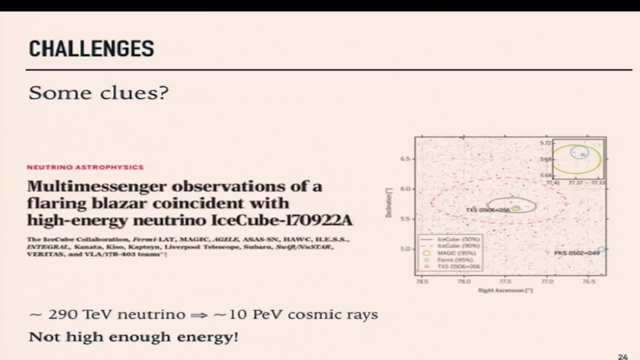 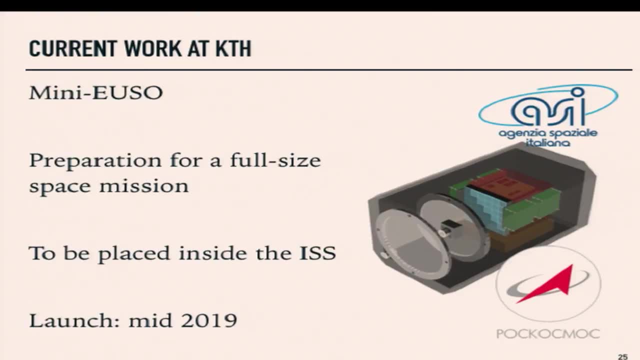 So it's still not quite high enough to be ultra-high energy, but still very interesting and probably more work to come on this in the future. So now I'm going to talk about the KTH work. So as a yeah, I should explain. 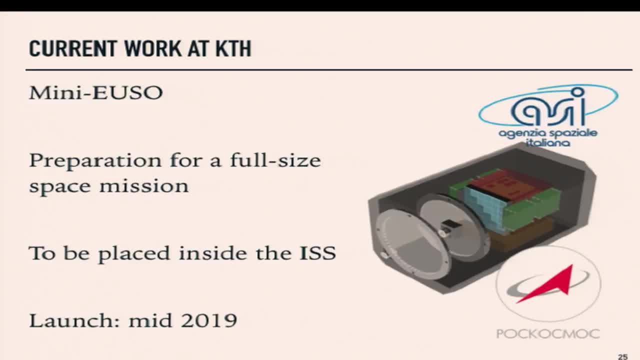 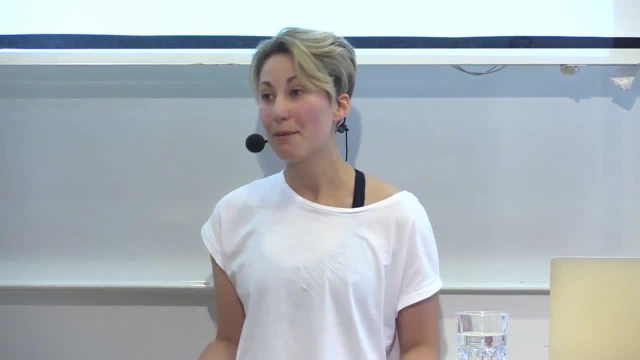 At KTH, it's essentially myself and my supervisor, who is Krista aka, the astronaut working on this project, But we are part of bigger collaborations so, like the USO collaboration that I mentioned, looking to do this detection. 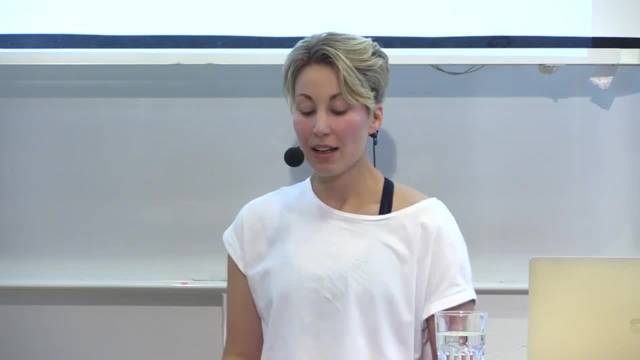 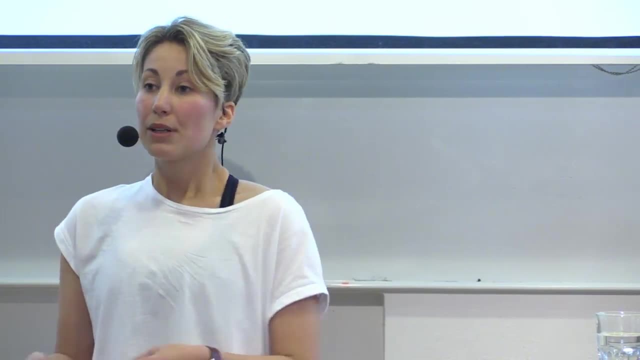 of ultra-high energy cosmic rays from space, And part of that project that we've really been focusing on is the building of a pathfinder detector, Because obviously, if you want to take a ground-based technology and put it in space, it's really challenging. 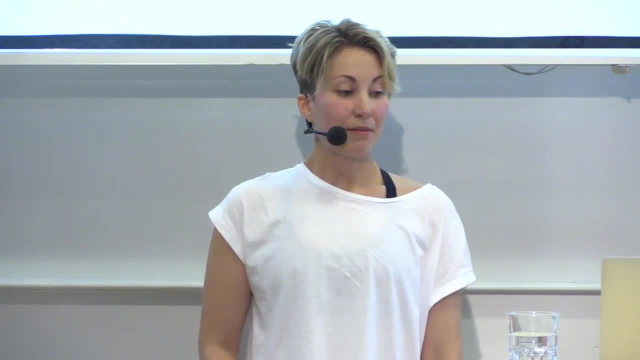 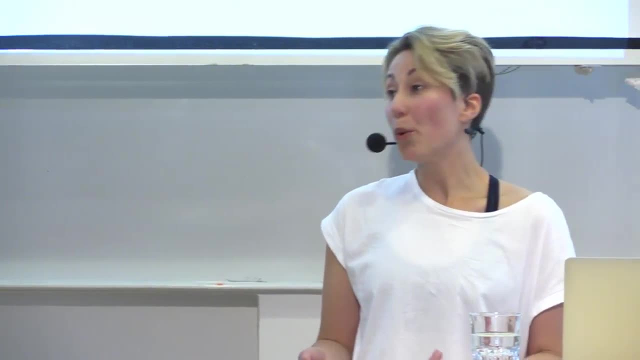 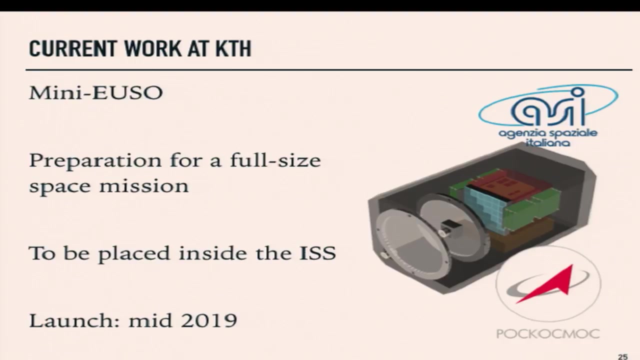 from an engineering perspective, If something needs to be much lighter, it can only draw so much power. it has to survive launch and so on. So what we're doing is we've built this small pathfinder and that's going to be placed. 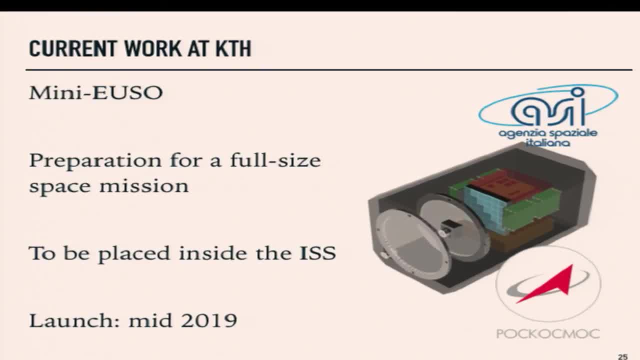 inside the space station as a kind of precursor for a bigger detector that could go outside the space station, And the launch for this is now planned for the middle of next year. So this instrument's probably going to be too small to really be able to contribute to the measurement. 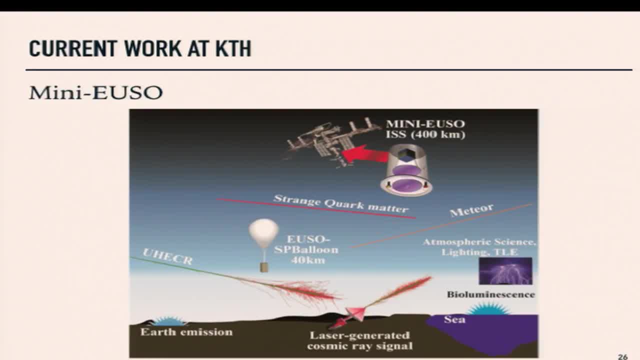 of the ultra-high energy cosmic ray spectrum, But it will do the very important job of characterizing the background from space. If we're going to try and look for these rare extensive air showers, we need to be able to recognize what kind of signals could be producing. 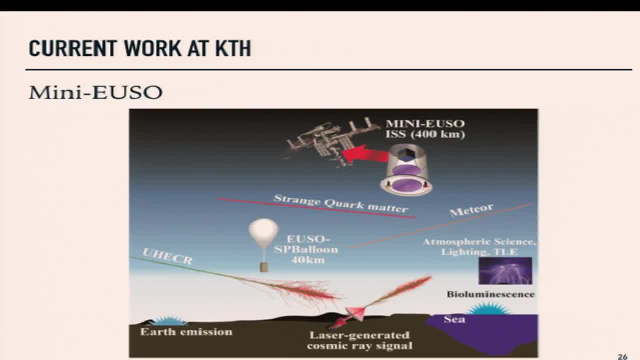 noise in the detector And, as is often the case in science, signals that we consider noise are very interesting to other fields, like meteors, for example, and upper atmospheric lightning. So there's also a lot of opportunity for lots of interesting. 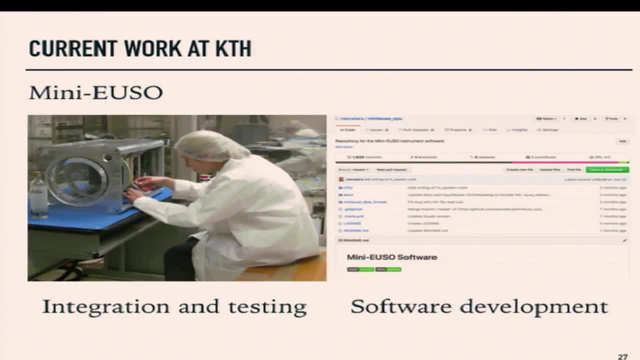 interdisciplinary science with this data. So the contribution has really been in the building and the testing of the instrument and also, in writing, the data acquisition software. So both of these things will go forward to larger projects in the future And the stage that MiniUSO is now at. 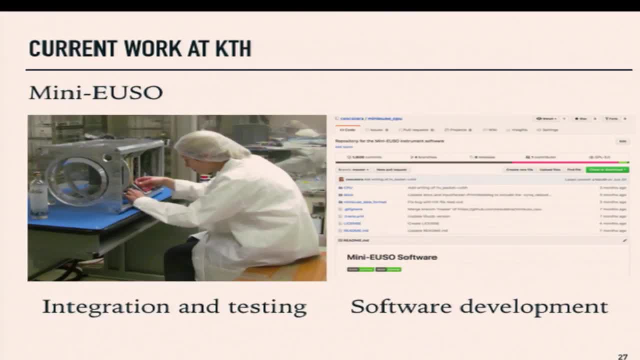 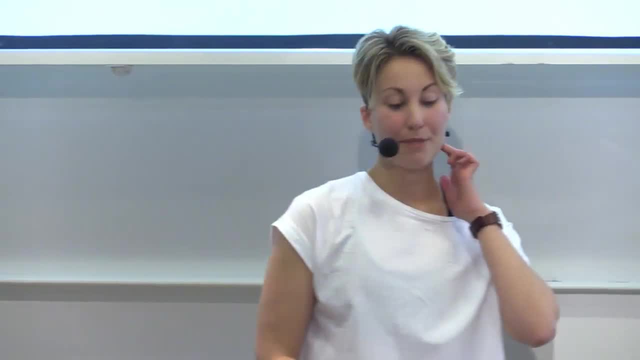 is that it's been built and the software has been tested, and we're looking to now space-qualify the instrument. It has to undergo a set of tests before it can be launched, And this is done by industry, so I get a little break. 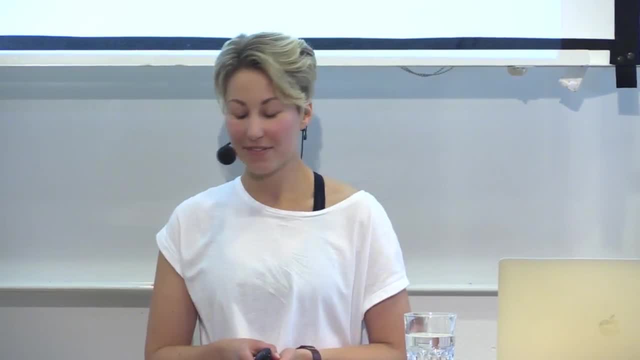 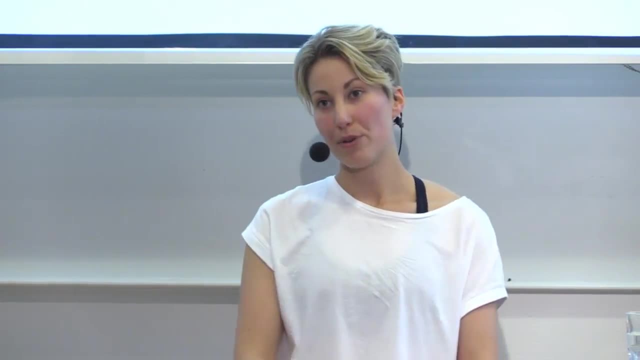 And in this time, with my PhD, I've turned to kind of think about: whilst USO is a very interesting project, it's very much a long-term project. We don't expect to be able to launch a giant instrument in the near future. 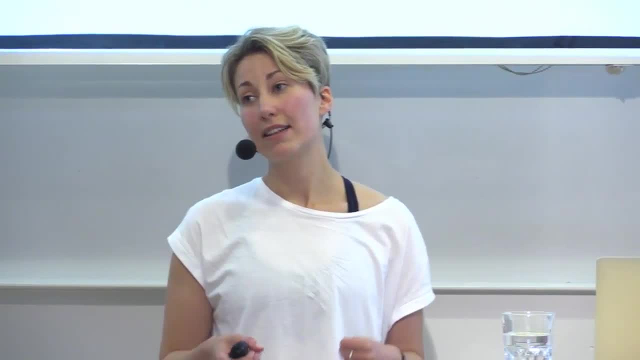 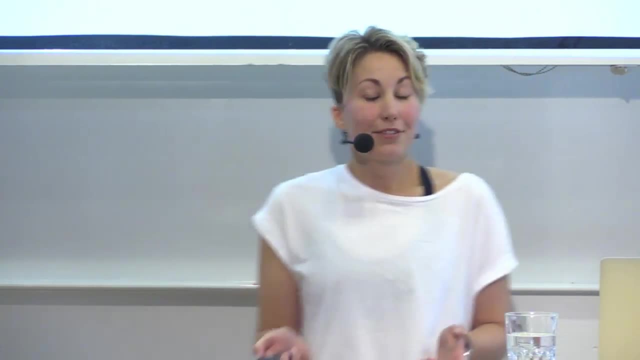 And we actually already have quite a lot of data at Ultra High Energies, And so I think it's interesting to look at this data in more detail And kind of try and figure out what we figure out something from what we already have. 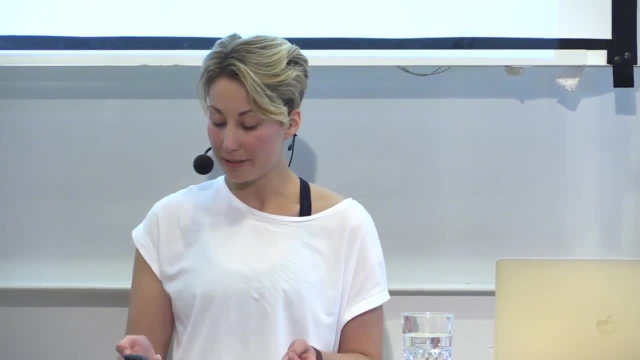 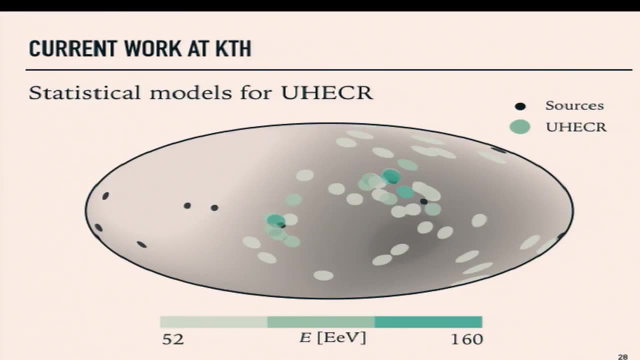 And this can be useful for informing future work as well. So something we're focusing on now is building statistical models for Ultra High Energy cosmic rays. So what this really means is just trying to fit a model to data so that we can compare what we think we know. 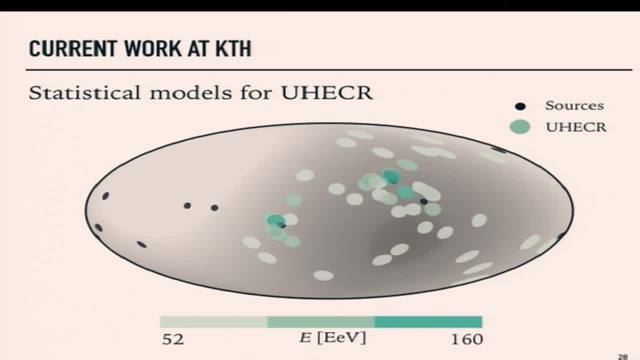 about the physics kind of the phenomenology that I've been through to, the data that we can see, And this is just a simulation which kind of shows the kind of information a model could contain. So this is a sky map in galactic coordinates. 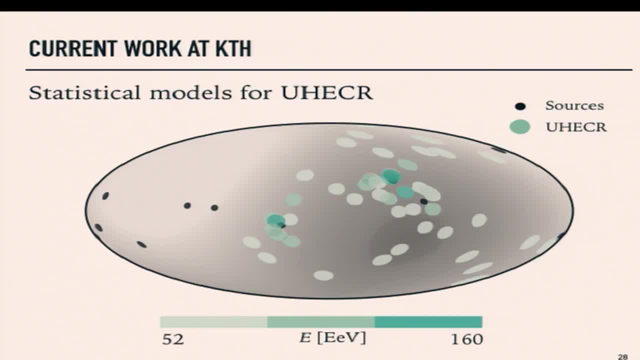 And these little black blobs are sources or a potential source catalogue, And these are kind of Ultra High Energy cosmic rays And the darker ones correspond to higher energy events. So here we can see that we kind of expect those to be less deflected from sources. 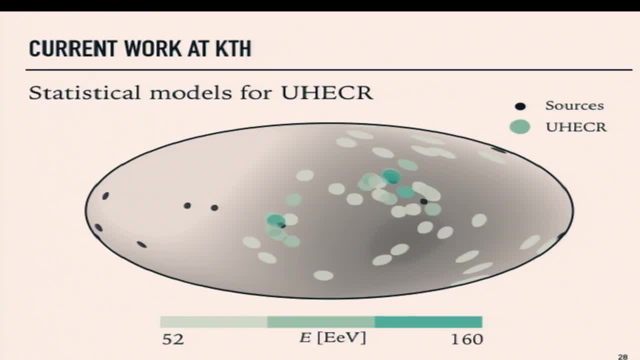 and to cluster around them, And then the lower energies, the lighter coloured ones, can spread all over the sky. So not so useful for doing astronomy, but still containing some information. And then this grey scale here is really just to show that there are detection effects. 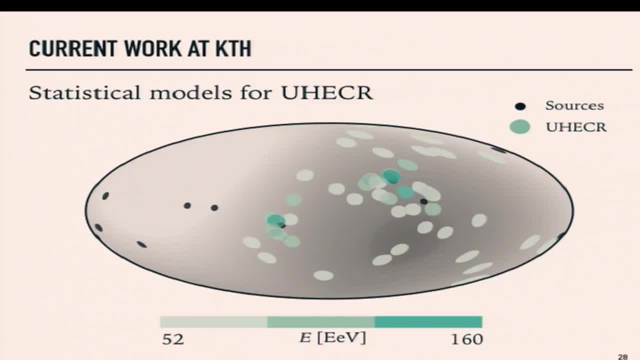 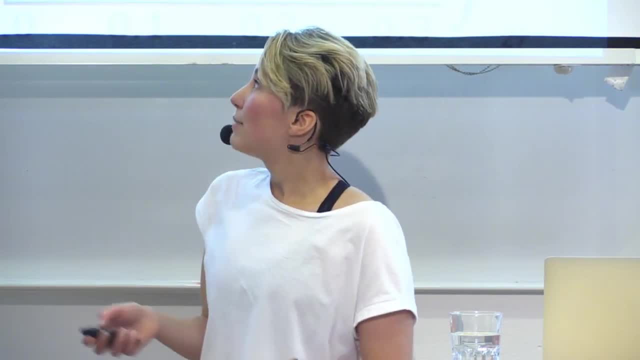 that need to be taken into account. The ground based observatories don't have a whole sky exposure and they have this kind of gradient depending on where in the sky you look. So this is something we've been doing, and the idea is to compare a potential source catalogue. 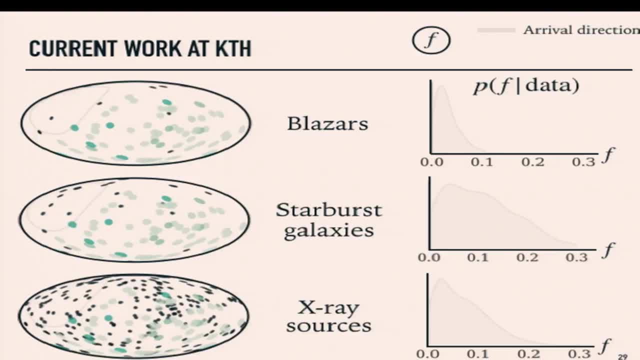 with the Ultra High Energy cosmic ray data and just figure out statistically. is there any connection between these two catalogues? And that's something that I've quantified here with the parameter F, which is just the associated fraction of cosmic rays with potential sources, We've got blazars. 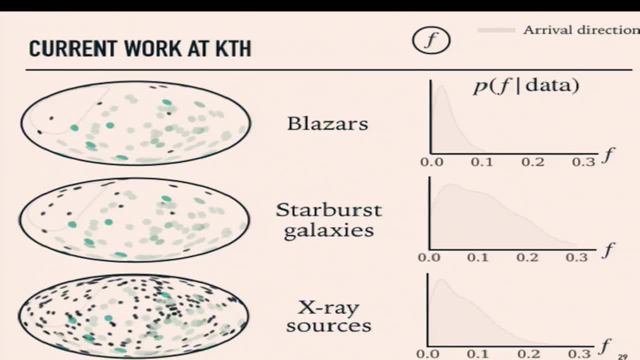 very popular right now thanks to the neutrino detection, Starburst galaxies and X-ray sources, And all of these catalogues have kind of been cut so that we only look in the nearby universe, where we expect to be inside the Giza-K horizon. 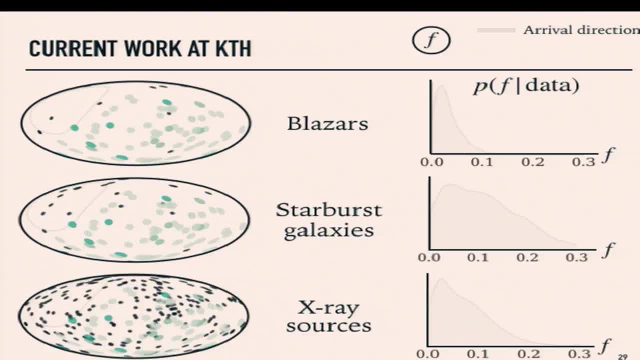 And then what we see is, if we just look at the arrival direction- so look for clustering in this kind of three-dimensional space that I can't really plot here- We see that there's not much connection. We have very low percentage associated with sources. 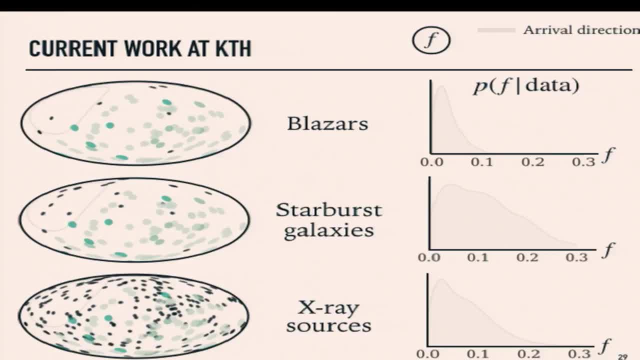 But maybe some hints. up to 20% of the cosmic rays could be explained by certain sources. But then the problem is that if you also take the energies into account, this really disappears. So I mean we've got these very high energy events over here. 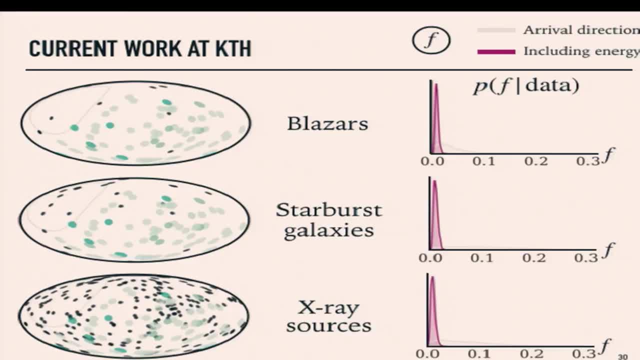 and we know they can't have come very far because they would have lost their energy And they can't be very deflected because they're higher energy, so they can't. the same magnetic field cannot deflect them much, But they've got no kind of sources nearby. 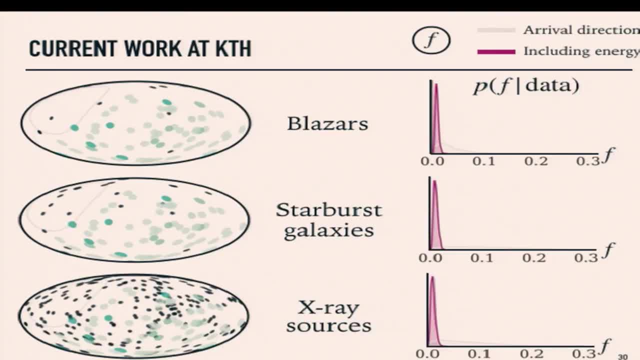 or here the ones that are. they're far too far away to explain ultra-energy cosmic rays of that energy, And so there's still a lot of kind of work to do here in bringing together the phenomenology with the data, and I think that's the kind of exciting part. 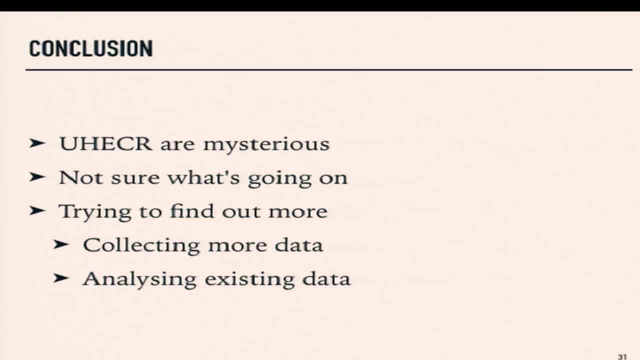 of the field to work in as well. So I'm going to conclude here. Ultra-energy cosmic rays are mysterious. There's a lot of stuff going on that needs to be modelled and so very interesting from physics perspective on all different scales, from source physics. 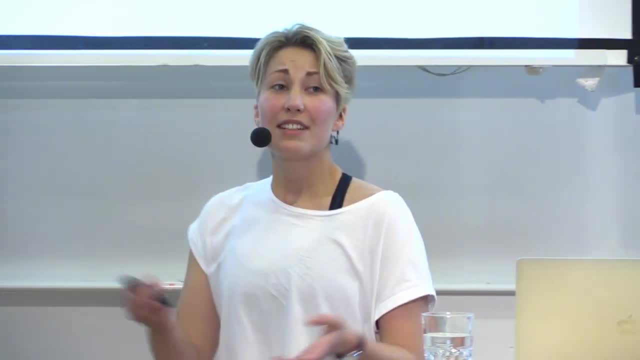 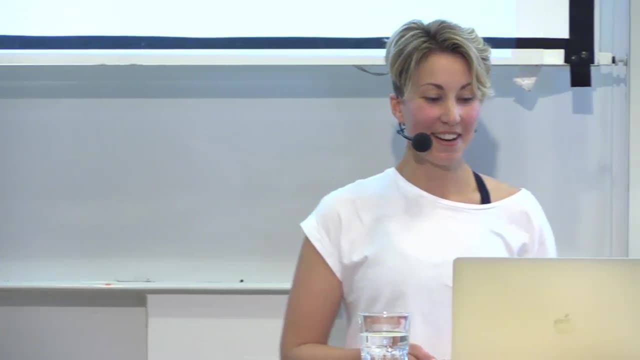 at very high energies to this kind of propagation and even detection, all the atmospheric physics of air showers and the reconstruction. So we're not still not sure what's going on, but trying to find out more and kind of two of the ways we're doing that at KTH. 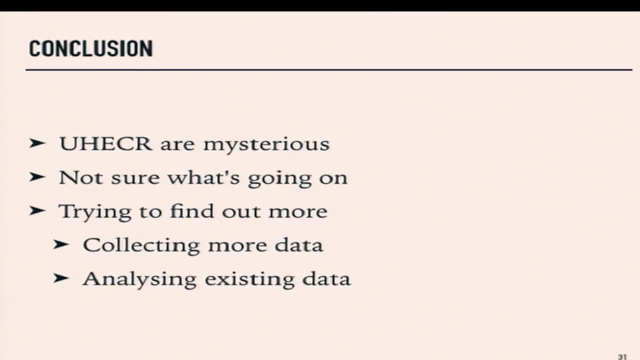 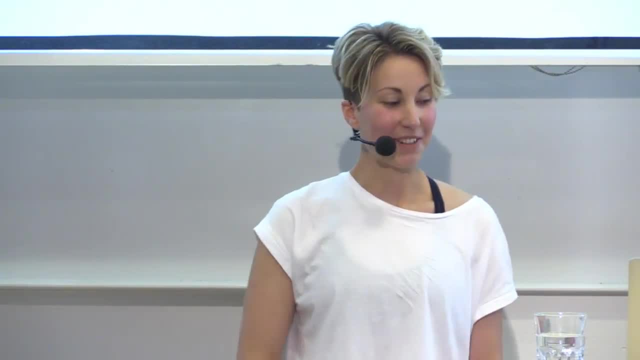 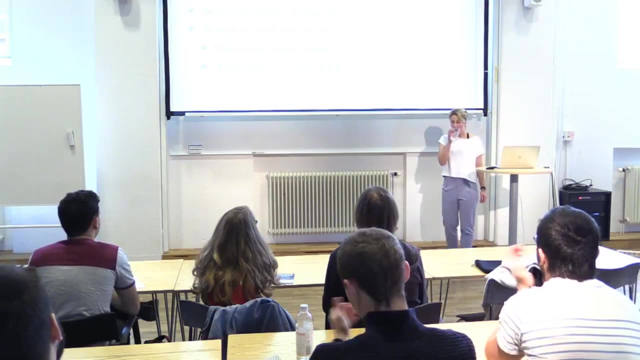 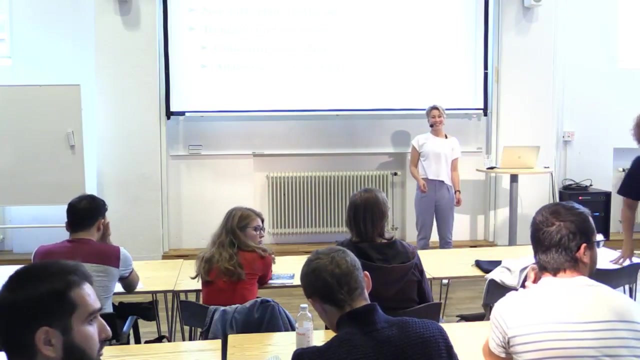 is building future projects to collect more data and then, while we're waiting for that, more data building analysis techniques to make the most of what we have. So, thank you. Do we have this box? I'll let you do the throwing First of all. 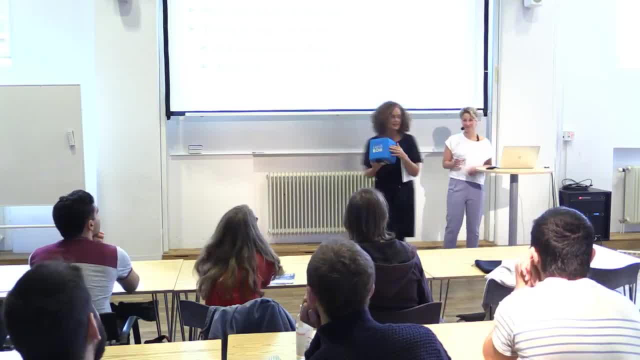 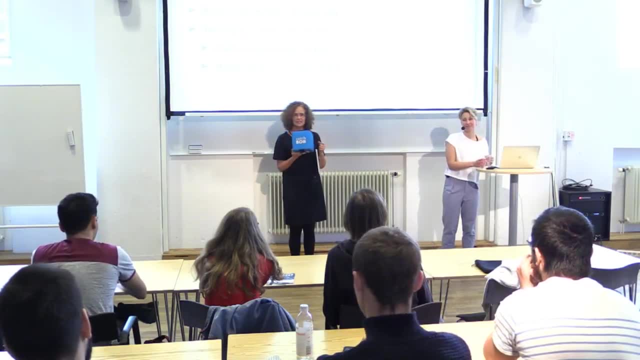 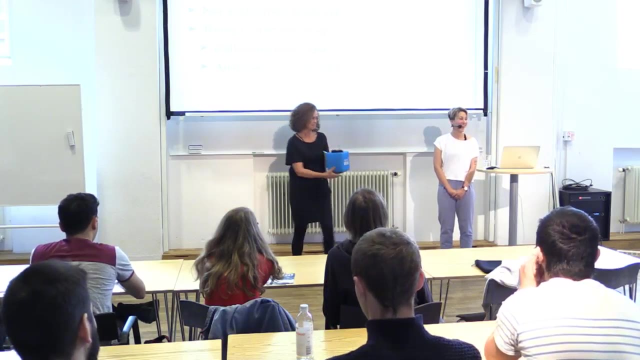 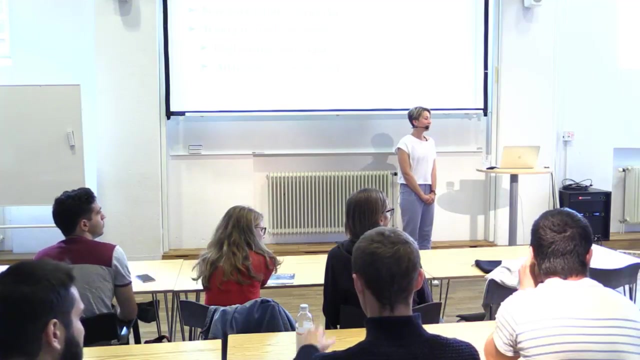 thank you so much, Francesca. What an interesting work you have. It's never boring. Is there anyone who has got a question for Francesca? Yeah, Don't be shy. Hi, I'm like I don't have any background. 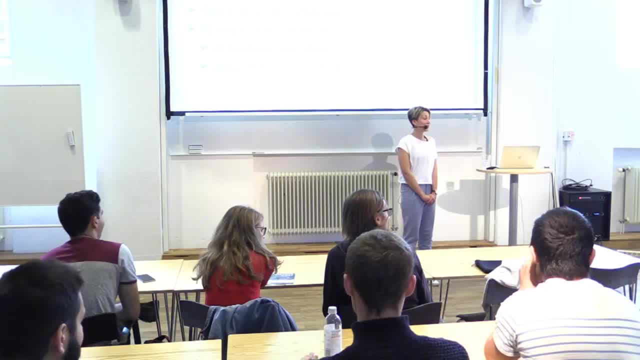 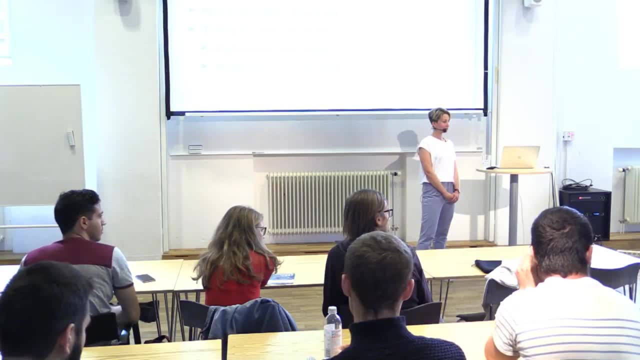 in ultra high energy cosmic rays. It's not unusual. But yeah, I was more interested in knowing, like the data you collect from it, Like what can you interpret from it, Like you mentioned the example of blazers, What more can you get from data? 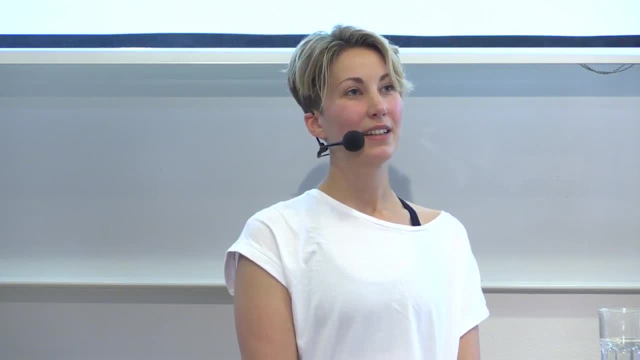 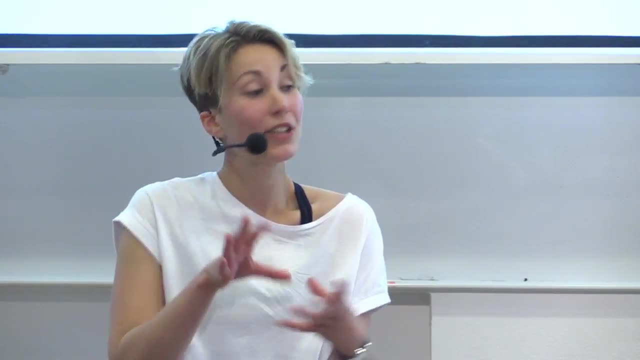 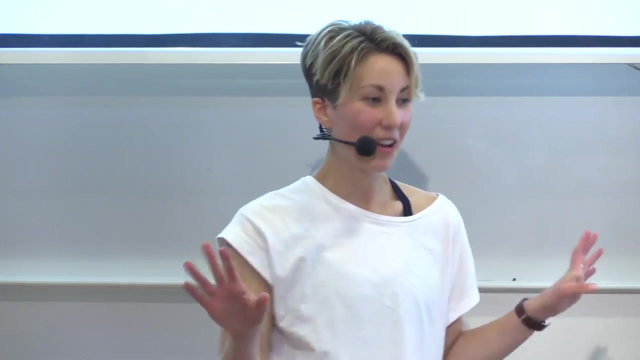 So I suppose what you can get from the data that is maybe a little bit more certain. I mean, it's still very much under interpretation, So all you can do is really constrain the possibilities So you can say, okay, it's not these kind of models. 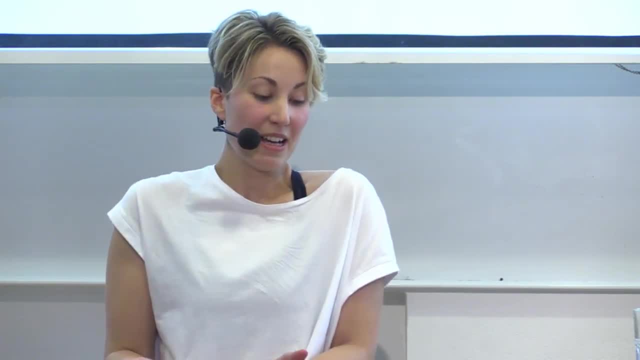 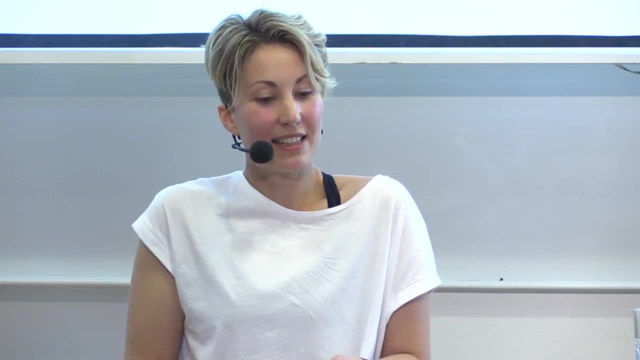 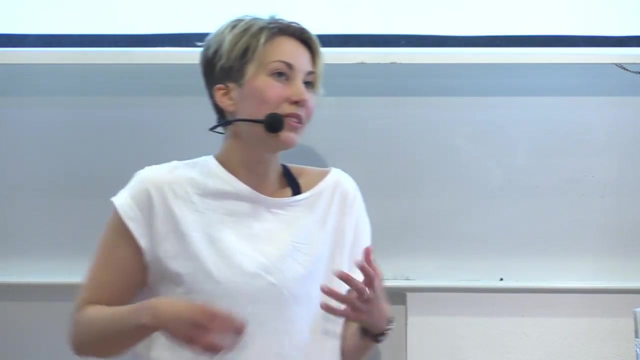 but these are still kind of open And the whole idea is that, by kind of either having more data or kind of doing a more sophisticated analysis, is to make those constraints tighter so that you can really narrow it down to the models that can correctly explain what's happening. 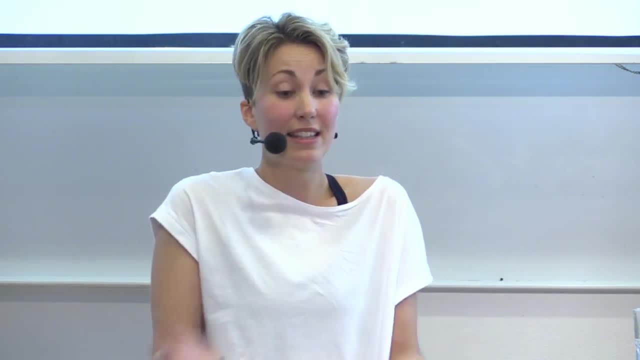 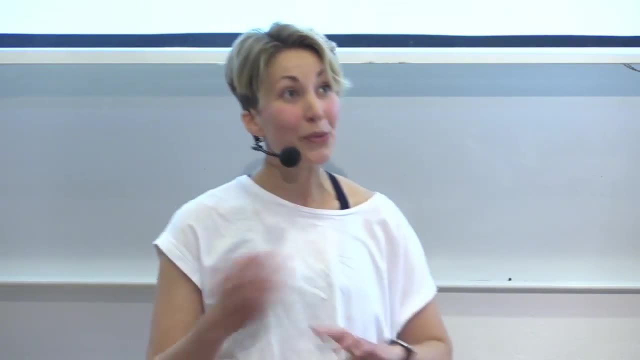 or even bring the constraints in, and you see that none of the models are working. And then you need to come up with a kind of very different hypothesis, So another. before the cutoff in the spectrum was observed, for example, people actually first hypothesized. 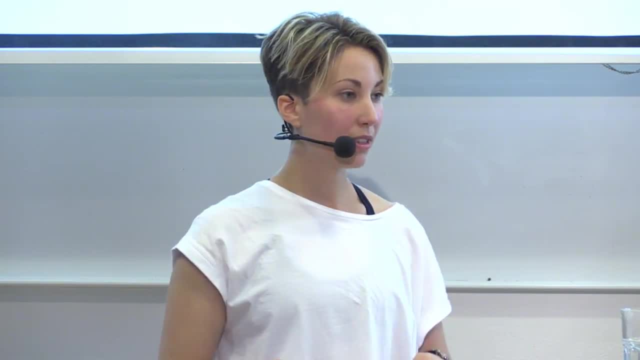 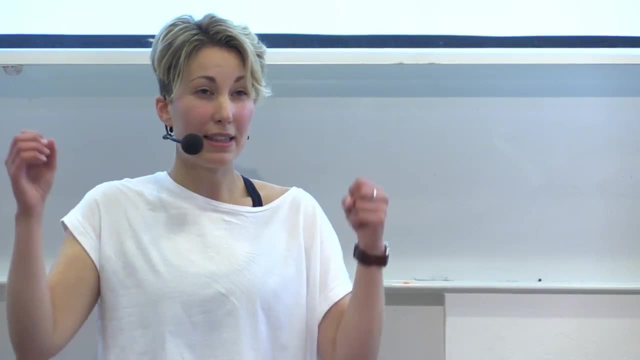 that there could be some top down process which produces the ultra energy cosmic rays. So, instead of being accelerated from low energies, they could actually be produced by the decay of very, very massive particles left over from, like big bang relics basically. So this was very much. 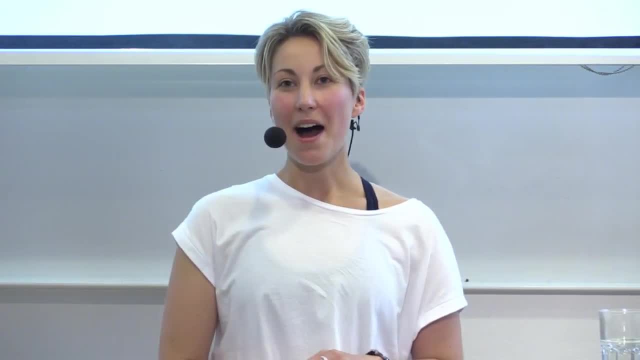 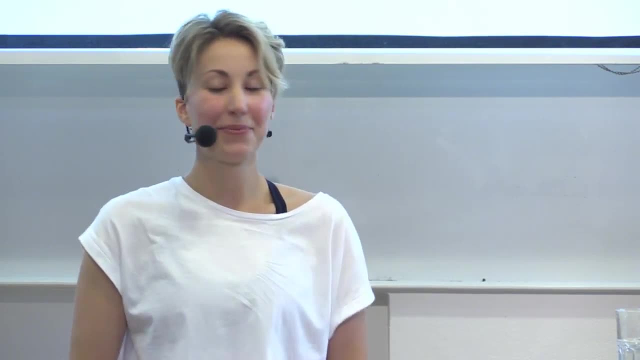 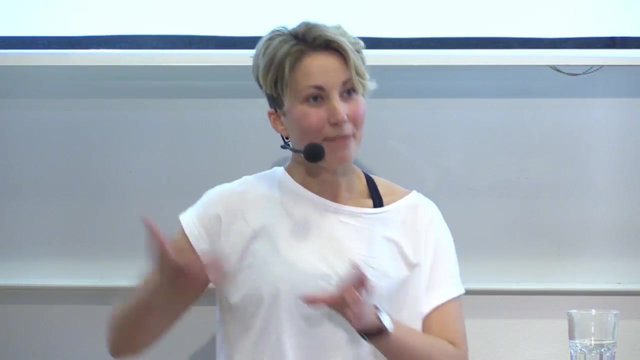 a kind of theoretical area of research. But since they observed that cutoff, that was really a motivation for, okay, we reach a maximum acceleration energy And these theories were kind of disfavored but still existing And in that sense it's also connected to the dark matter problem. 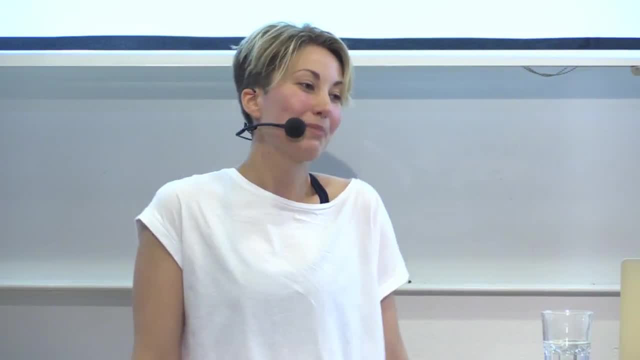 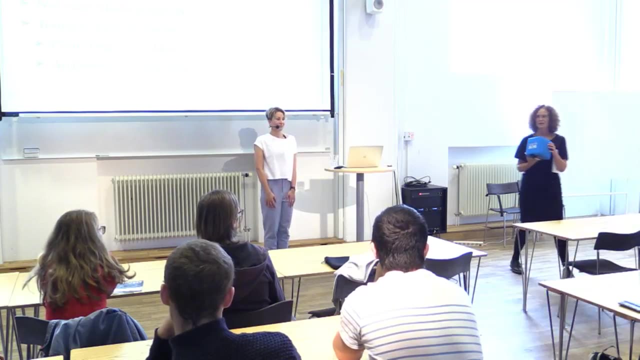 and cosmology. So it's a lot of interesting possibilities there. Yeah, Thank you. Anyone else? Yeah, Thanks for the talk. It's pretty interesting Question. You were talking about collaboration with TADR. I'm not sure if that's the right word. 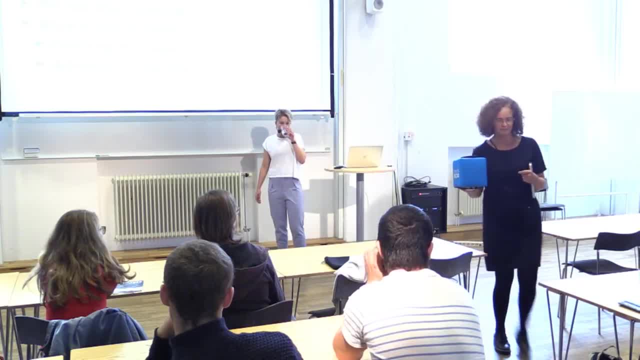 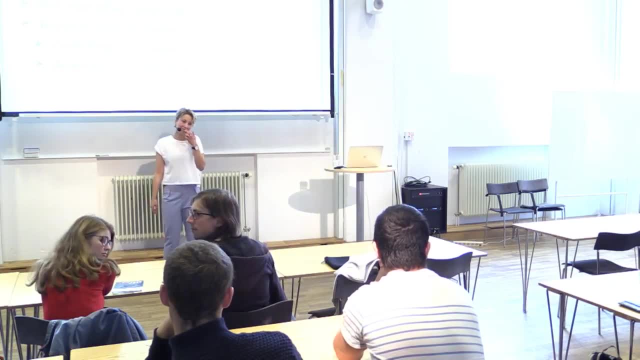 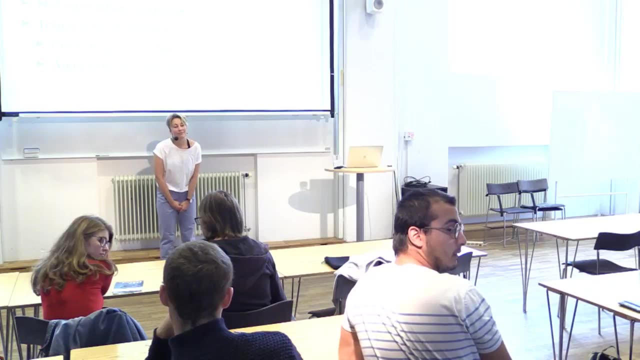 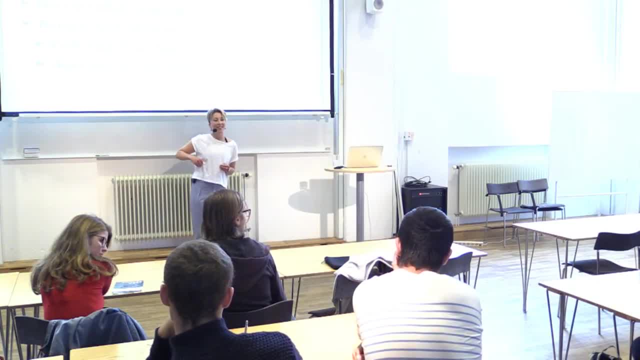 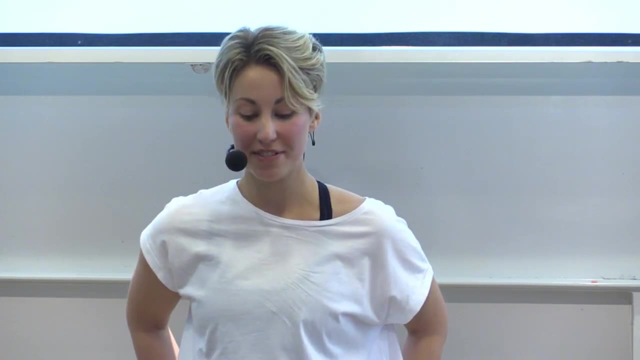 Yeah, thanks. Yeah, Looking at meteors and other stuff which you consider noise? Yeah, Is it at the moment just potential or are you actively researching? No, this is something we're actively looking into, So hopefully right now on the International Space Station. 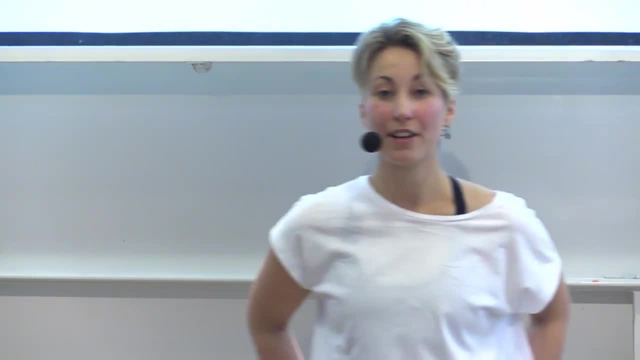 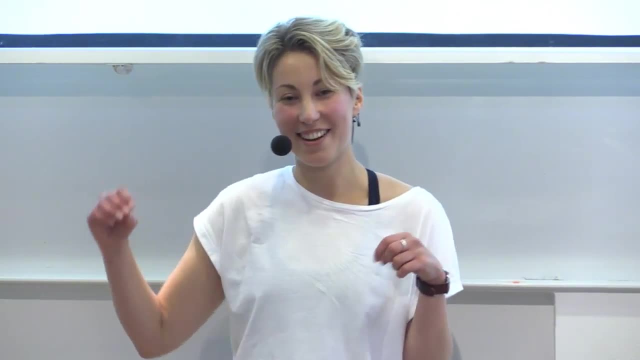 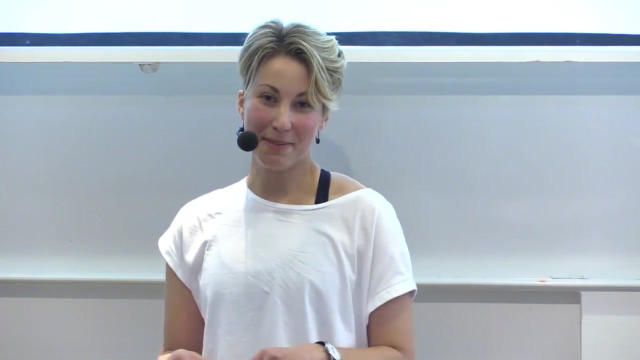 there's an instrument called ACIM, which was developed in Copenhagen actually, which is built to detect these upper atmospheric lightning, called transient luminous events, to study these in more detail, And we hope that they will still be on the space station at the same time that our instrument was there and that. 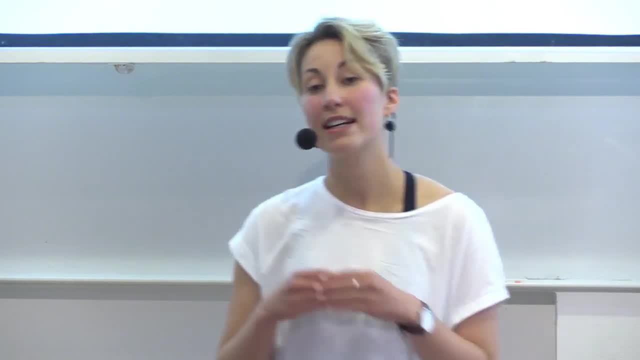 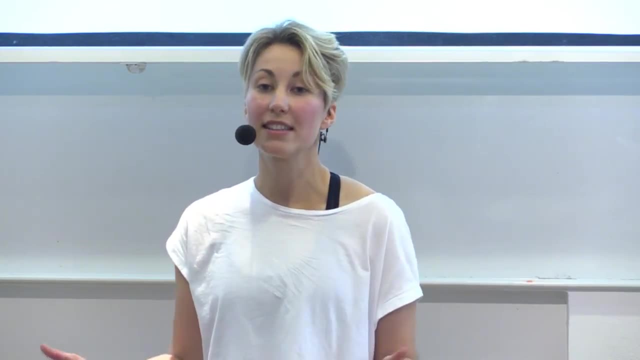 what we can give that their instrument doesn't have is a very high time resolution, because in order to observe these air showers, you need to have microsecond resolution, because they happen very fast, Whereas lightning is, believe it or not, relatively slow takes. 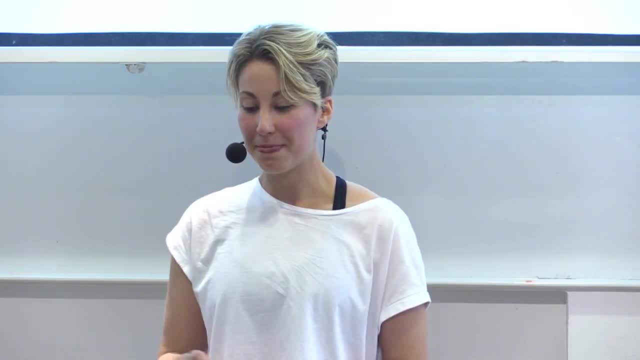 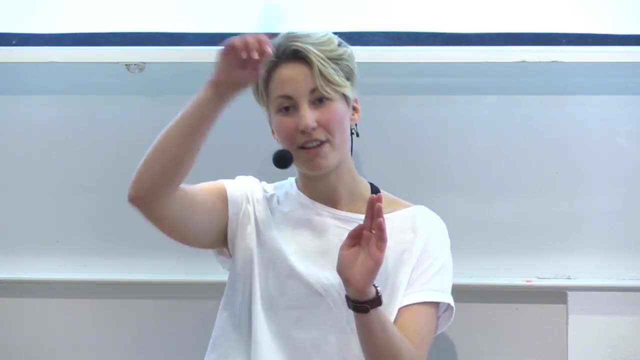 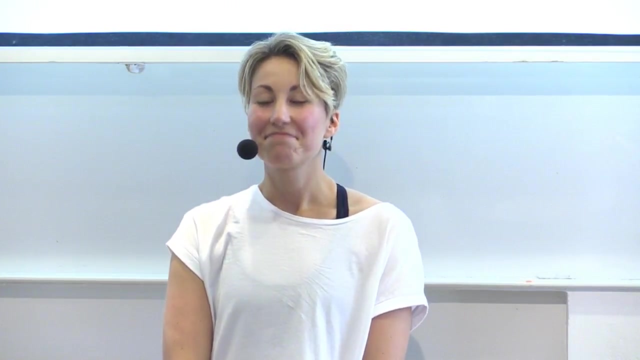 place on kind of millisecond timescales. So they're interested in our detection of the same lightning because we might have more detail in time on the rising phase, which is not so well understood from a plasma physics perspective. That's one example. 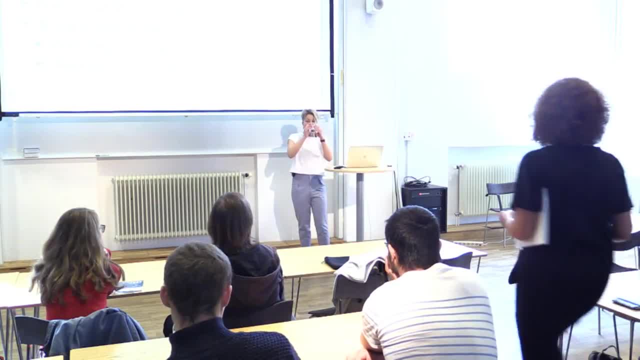 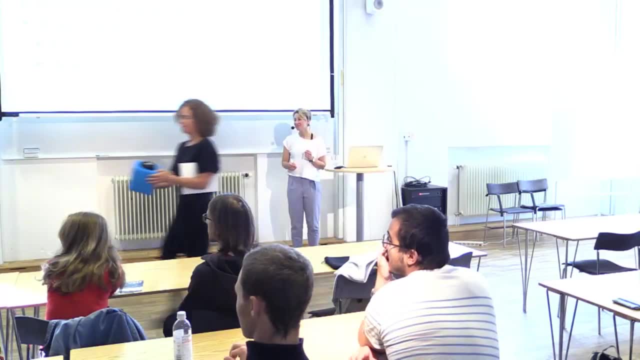 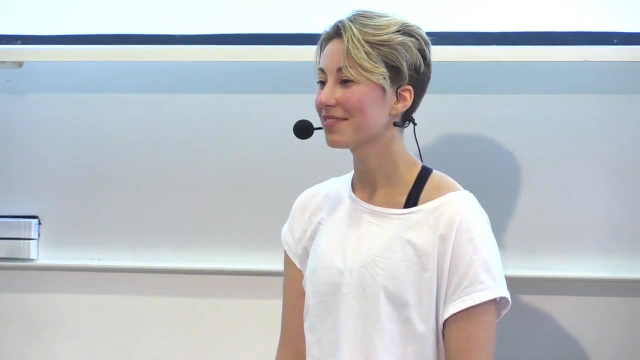 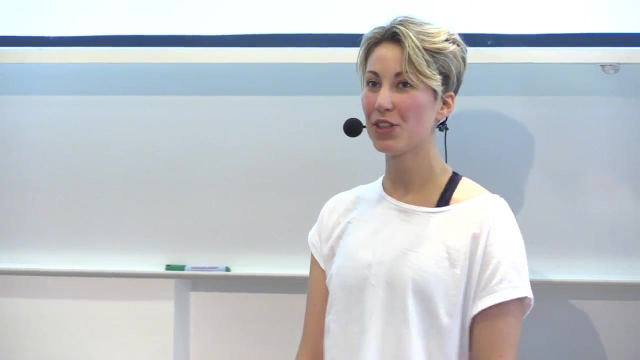 Maybe very basic, practical questions. How long do you have to sit in this observatory to actually see one of these air showers? Right, yeah, so to get a feeling for it, the two detectors have now been operating for about 10 years, But I mean they've been growing during that time, So it's a very, very long. period of time, But I mean they've been growing during that time, So it's a very, very long period of time. But I mean they've been growing during that time, So it's a very, very long period of time. So it's a very, very long period of time. So you'd, of course, run. 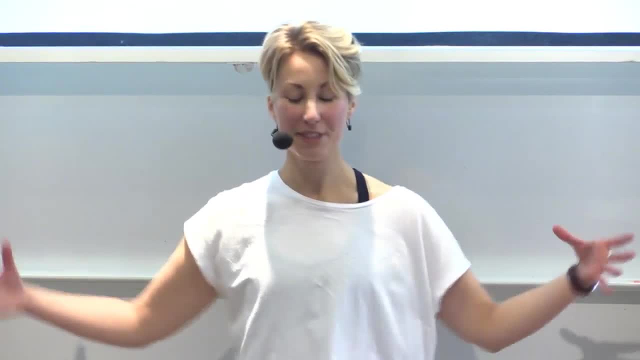 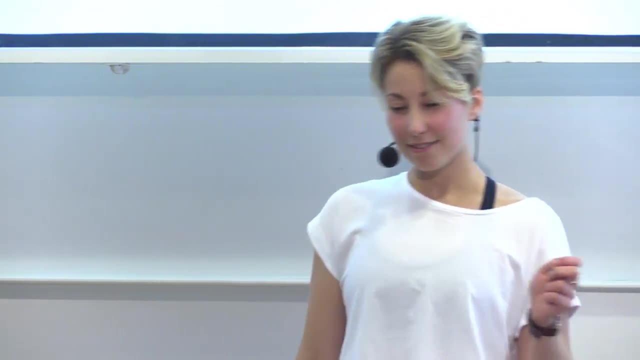 around that time. So you'd of course run around that time. So you'd start off with not a very big array on the ground and it kind of grows as you build and add more detectors And we have, let's say, some 500 events over the ultra high-energy part And we have, let's say, some 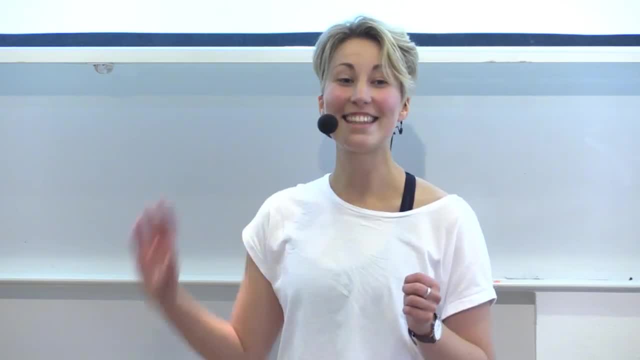 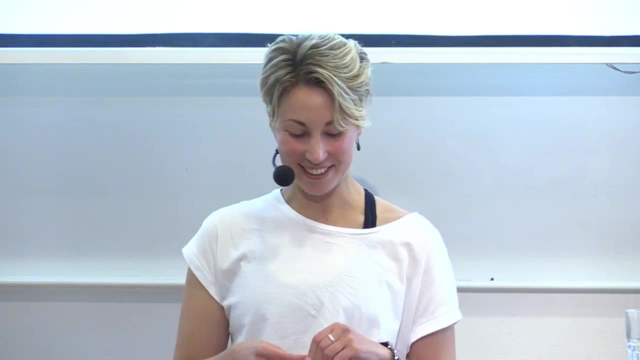 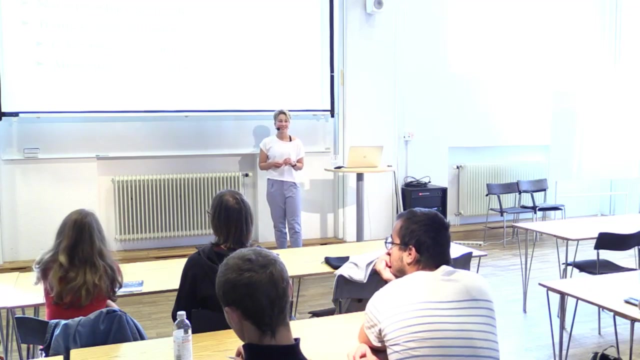 500 events over the ultra high-energy part. So it's really slow Even so. So that's the motivation for going in space right there. Yeah, Thank you. okay, no more questions. i'm getting hungry, so i'm also happy to chat afterwards, so 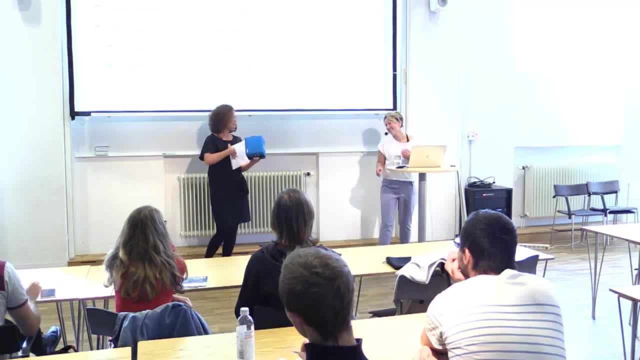 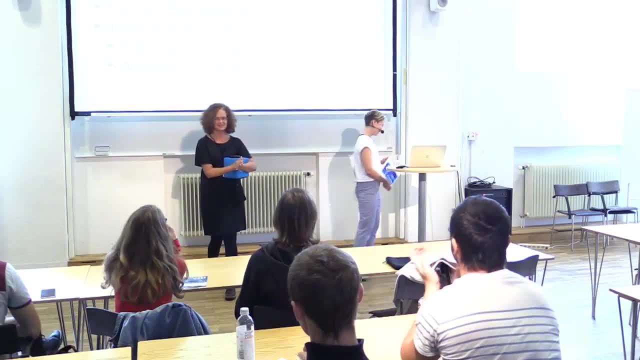 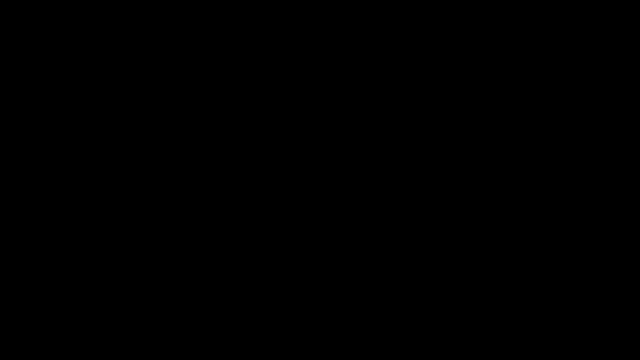 francesca: a small bit from us about not space, but art. thank you, i need more of this. yeah, thank you very much you.